two different axes. So what I'm going to do is rotate this function about two different 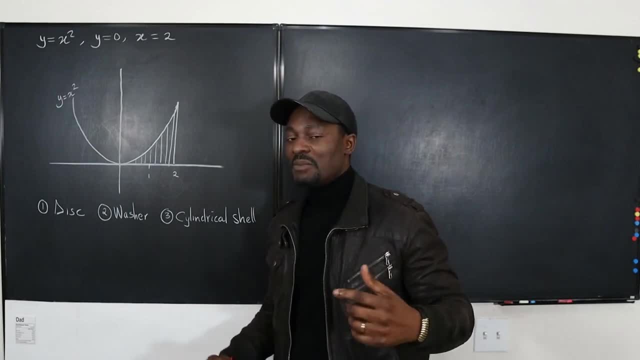 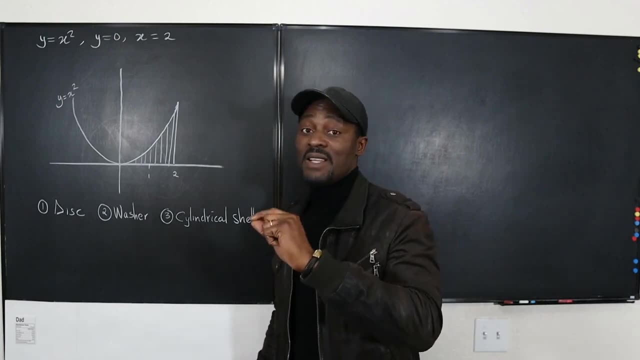 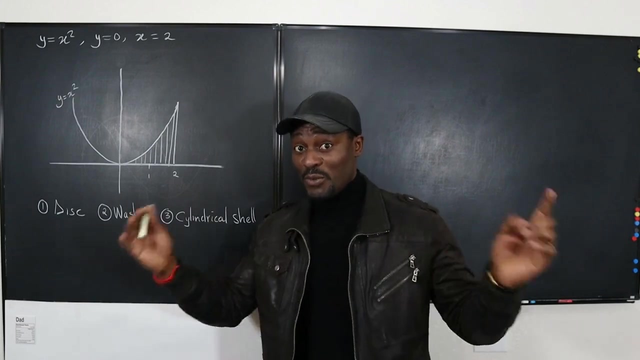 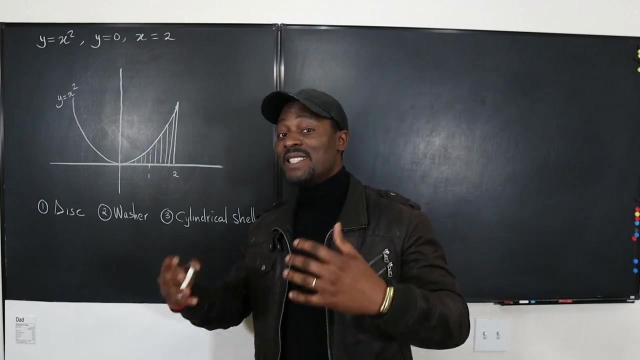 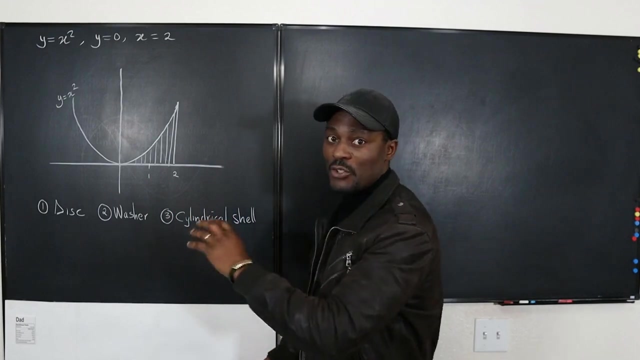 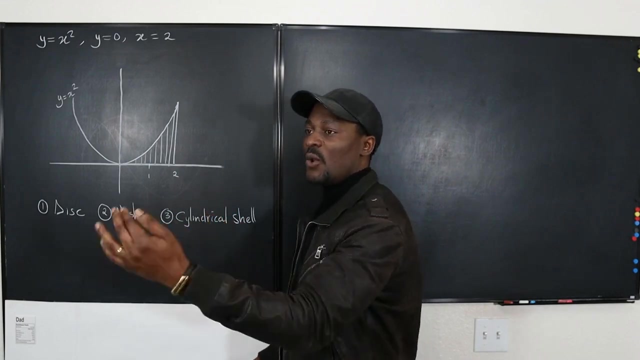 shapes. Now, one of those shapes is going to be something we can find using the washer method, and the other one is going to be something we can find using the disc method, okay? Now, whichever method you use, whether disc or washer, remember the universal one is the cylindrical shell. That's the one you should master, because the cylindrical shell will work even when the disc will not work, or when the washer will not work, okay? So, you want to learn it. So what I'll do is I'm going to do the disc and the cylindrical shell, then I'll do the washer with the cylindrical shell, or in reverse order, however, okay? So, let's get into the video. 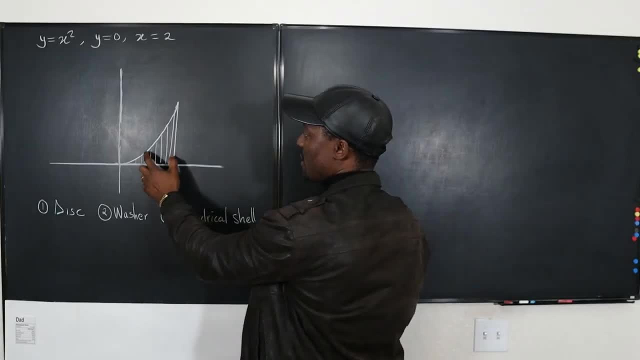 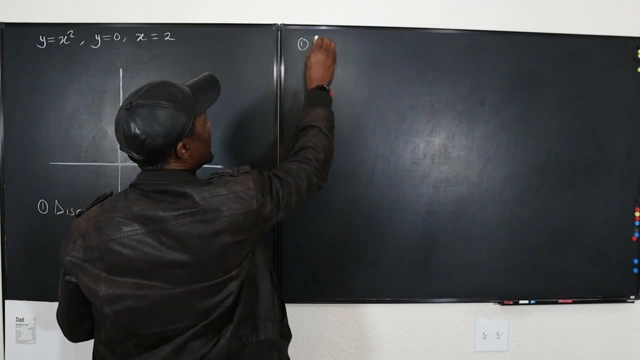 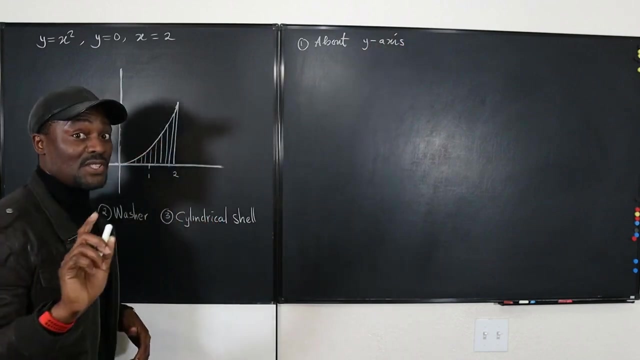 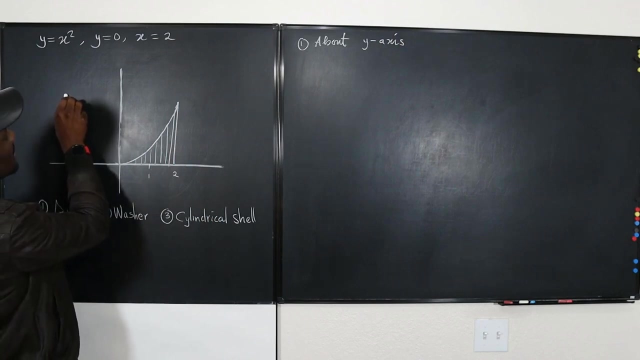 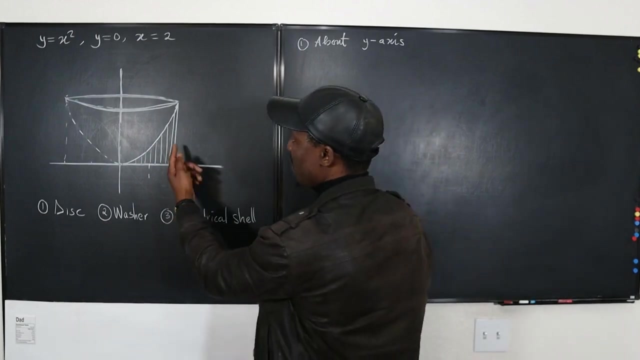 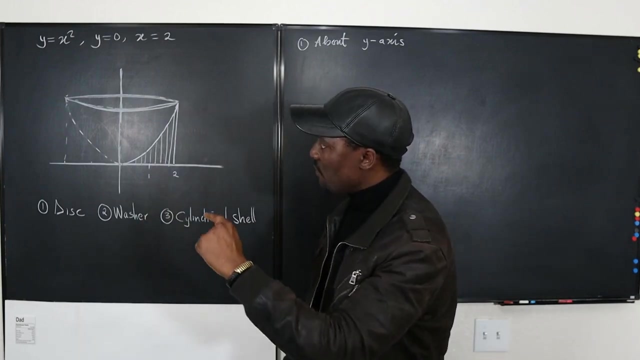 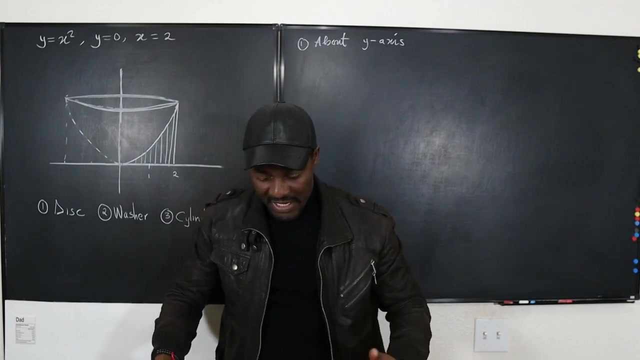 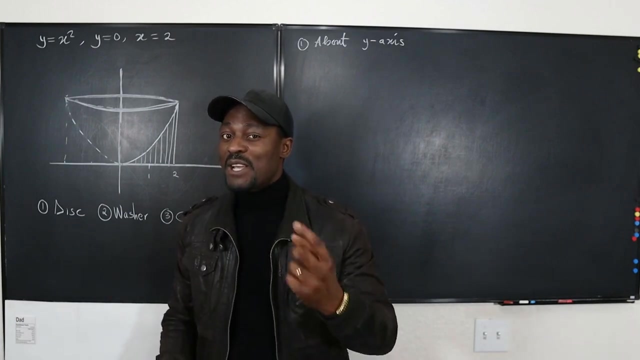 So, let's take the very first one. I'm going to take this, this solid, okay, this area, and rotate it about the y-axis, okay? So, let's make that the first one. Let's call it about the y-axis, okay? Remember, you have to be able to sketch whatever you're talking about. So, this is going to go as far out as here, so something like this. You need to sketch something that goes like this, okay? Something like that, and it's going to curl down. Like this, and so this is just all imaginary, okay? The real part that you're rotating is this, but you're going to have a shape like this, okay, if you rotate it this way. So, that's what we've got. It's a bowl, but the solid part of it is the lower part. So, it's more like a bowl that has a solid inside. So, if you want to find the volume of the solid that's generated, you'll notice that if you look into the bowl, it is thick on the inside because you can't go deep enough. This thing is going to keep stopping you. So, you have two radii. There's an inside radius and there's an outside radius. Those are the two things you need to identify. 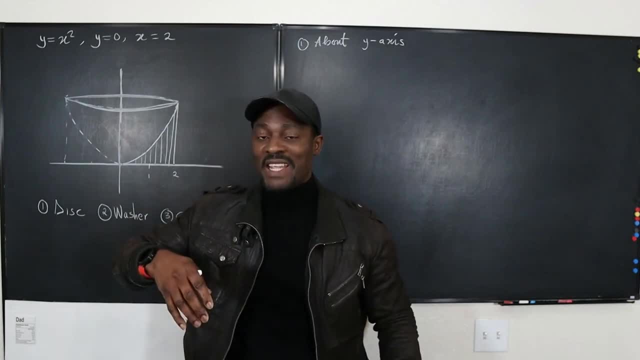 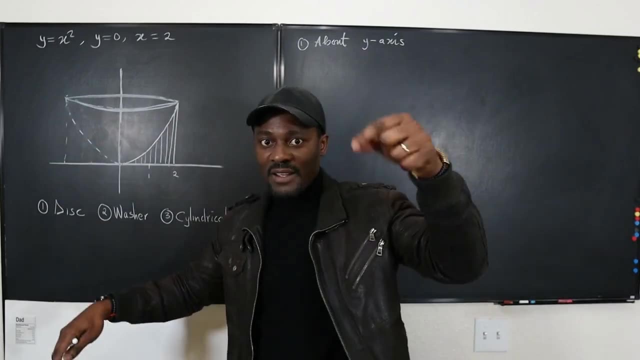 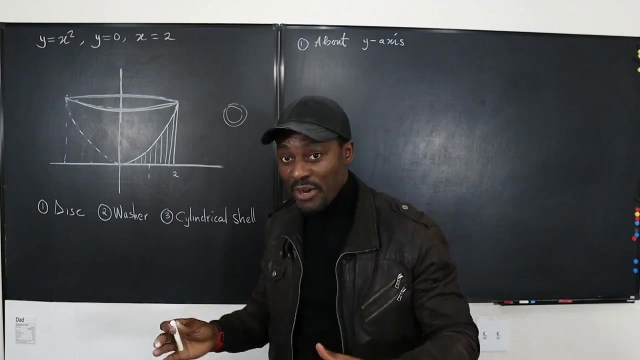 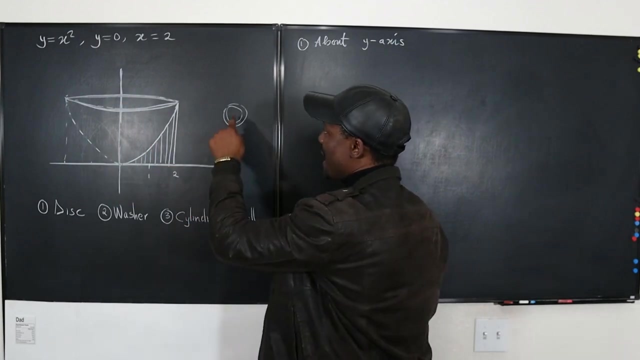 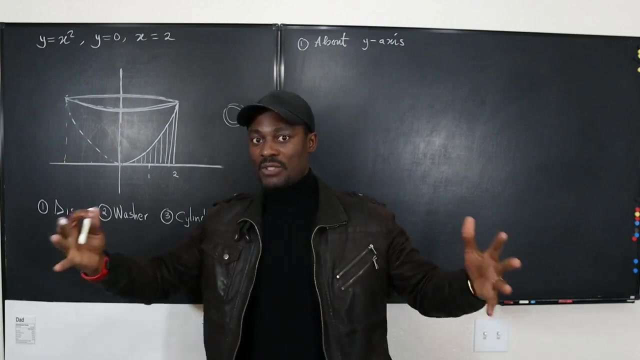 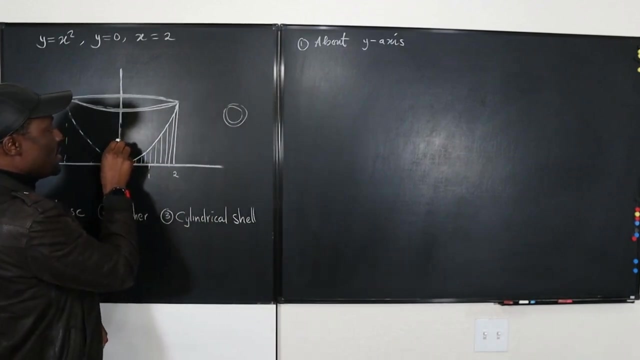 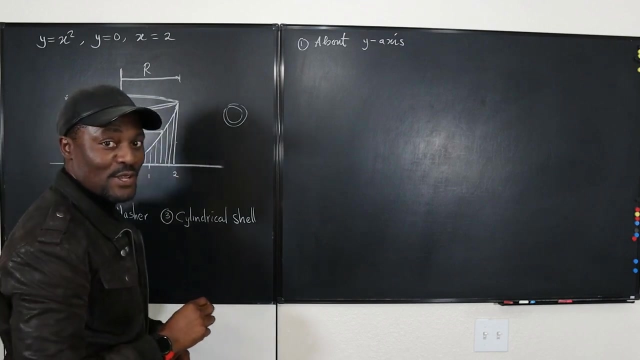 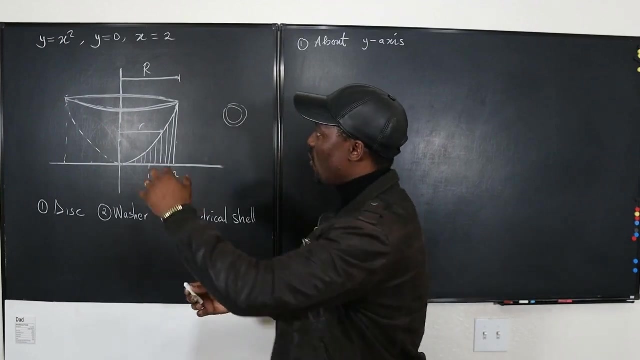 Because you have two radii, because there's a hole in the middle or a hollow in the middle, it is not a disc because if you slice this this way, you're going to get a washer. You're going to get something like this, okay? At every point, you're going to get a washer. At every point from the top until you get to the bottom of it. So, because you're going to get an inside radius and an outside radius, you just need to know what those two radii are, okay? So, the outside radius is usually the bigger radius, so we call it the big R. So, we're going to say the distance from here to here is the outside radius. You see this? That is the outside radius. And the distance from here to the inside here, at any point, is the inside radius. Okay, so remember, it's more like a cylinder that has been chopped out. Okay, so what do you call this area? It is just pi R squared but we have two Rs. 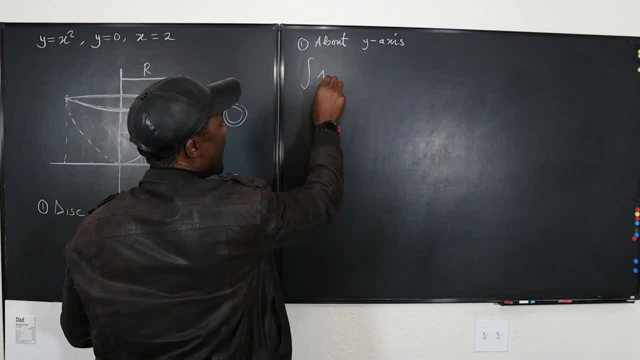 So, we're going to say our integral is going to be pi. Instead of saying R squared, it's going to be big R squared minus small r. So, it's going to be pi R squared plus small r. 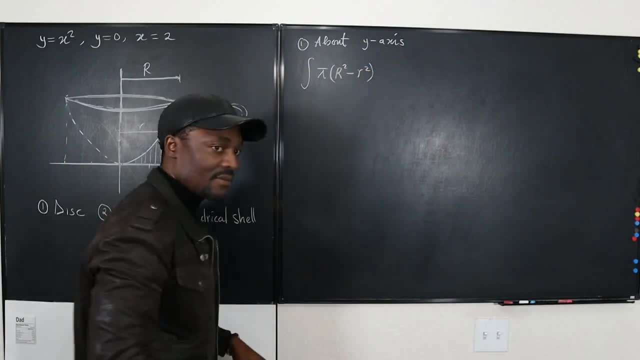 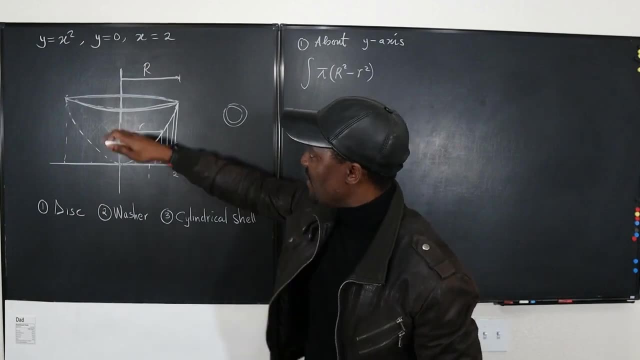 So, we're going to say our integral is going to be pi. Instead of saying R squared, it's r squared that's how we write it okay now is it going to be dx or dy remember that the thickness 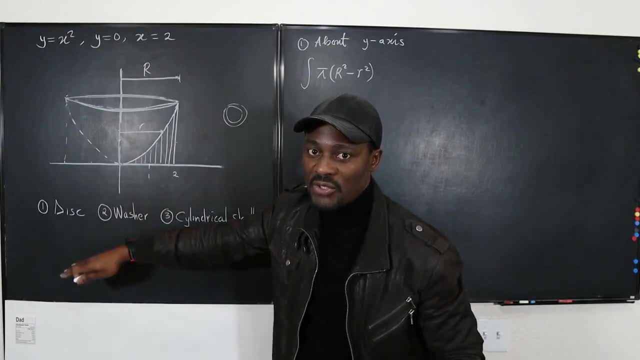 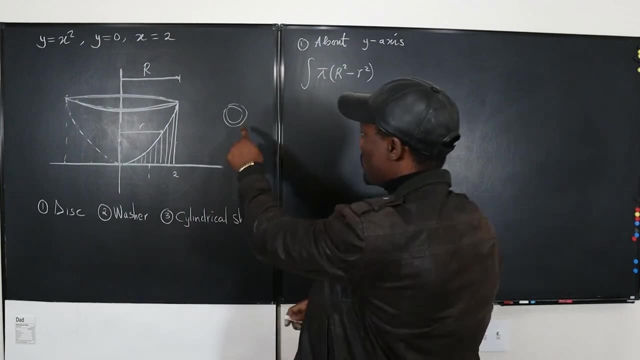 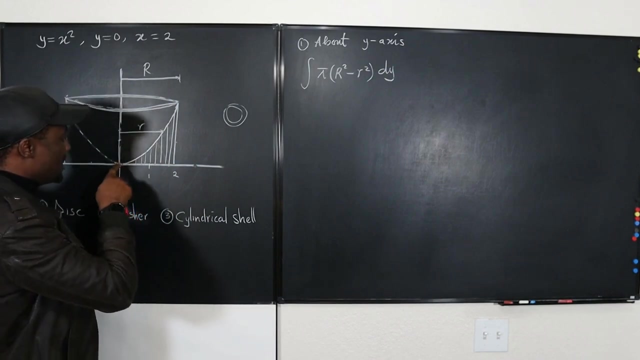 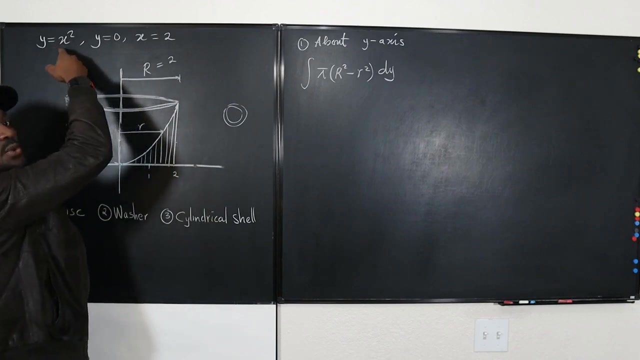 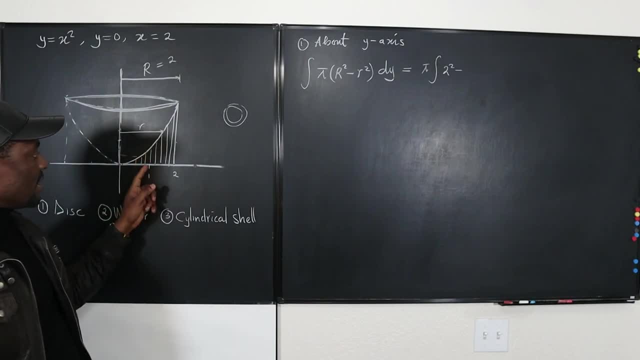 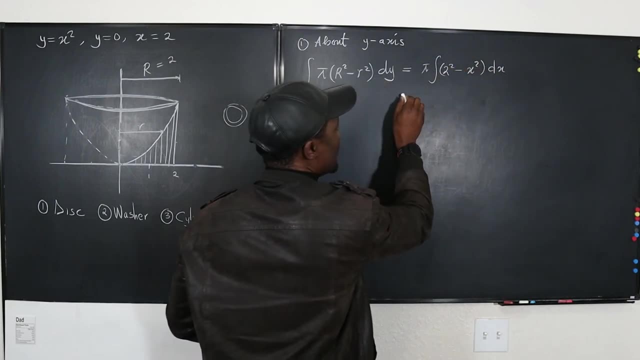 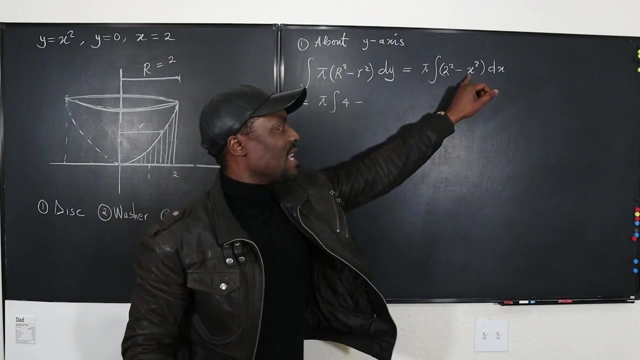 r is any value of x that you can read down here we're going to say it's going to be x squared and then we have dx and as you can see this is the same thing as pi times the integral of four minus now what is x squared based on what we're doing you cannot use x squared because i'm so 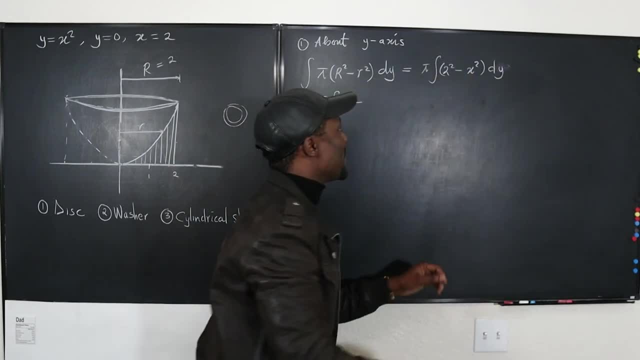 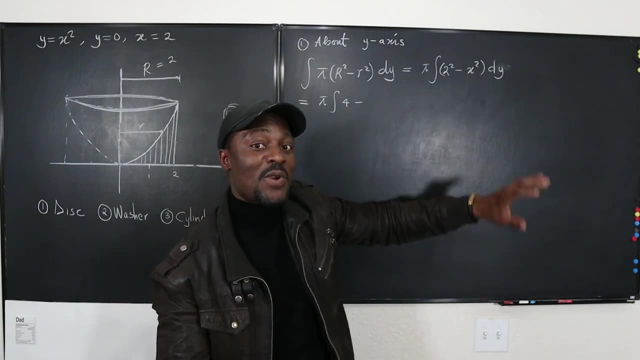 sorry this is dy okay dy so we cannot use x squared in this integral because we have to write it in terms of y so you have to change your x squared to write it in terms of y and what did 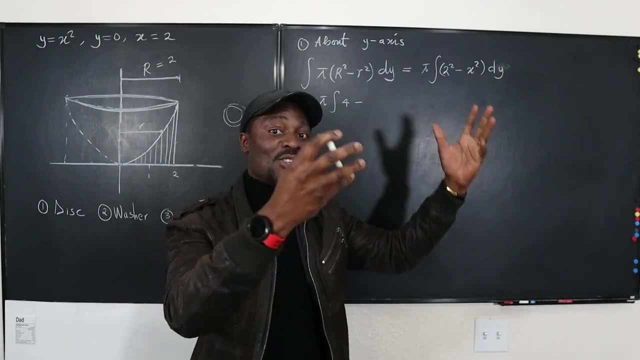 we say x squared was x squared is y so we're going to change this to y and then we do dy 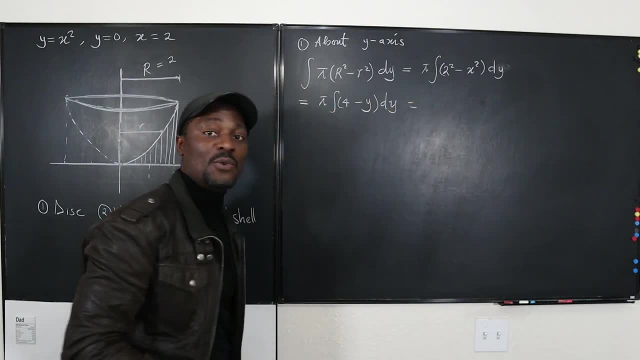 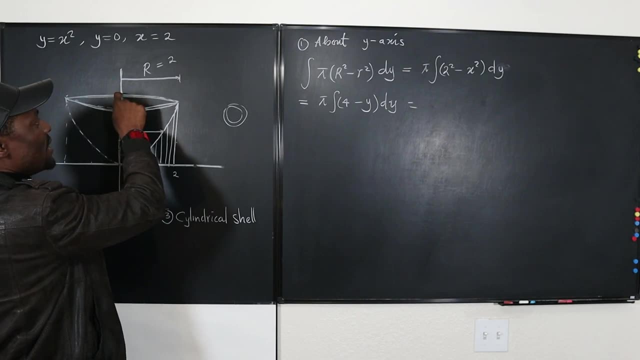 okay so now let's take the integral oh by the way what is the height we're integrating all the washers starting from zero to this point we need to know what this point is okay and that we can find this point just goes parallel to this point and this point is where x 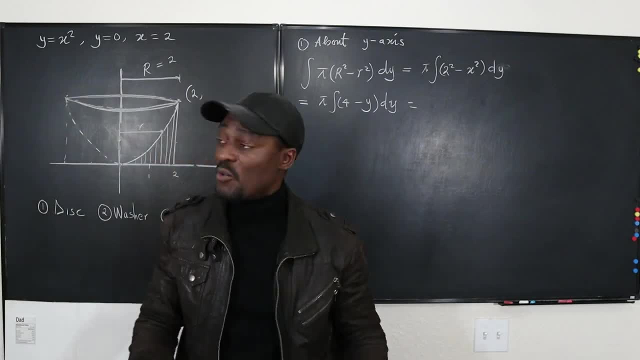 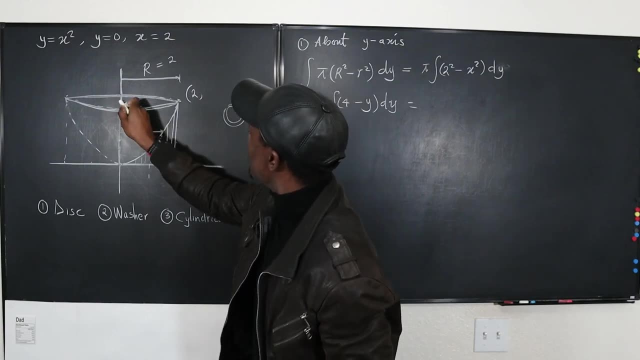 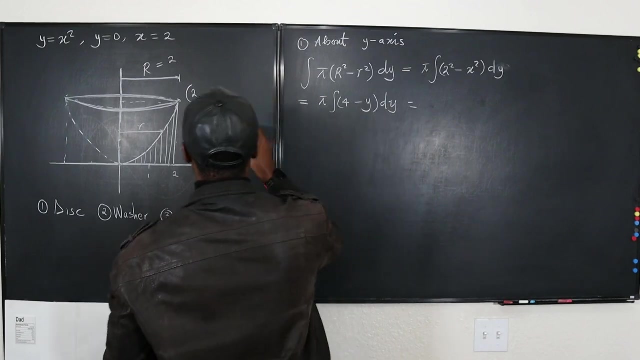 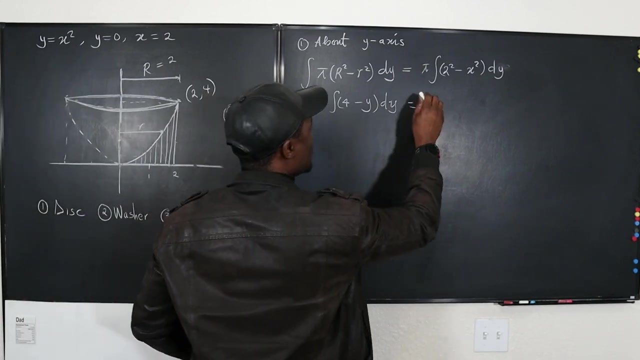 equals two let's go back to the functions we have when x is equal to two what will the y value be the y value is going to be hey this is it y is going to be 2 squared which gives us 4. so it's going to be 2 4. so the height of what we're integrating is from 0 to 4 and that's what we're going to do so this is the integral from 0 to 4 we should have done that a to b let's do it 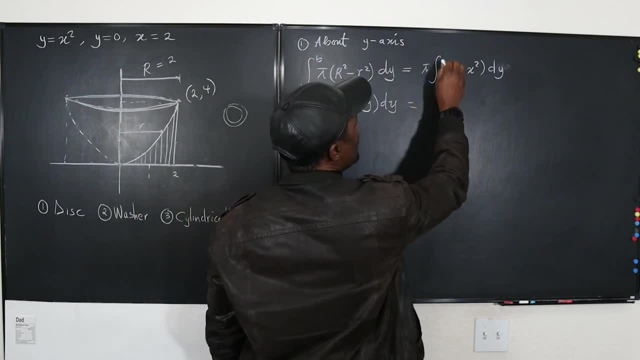 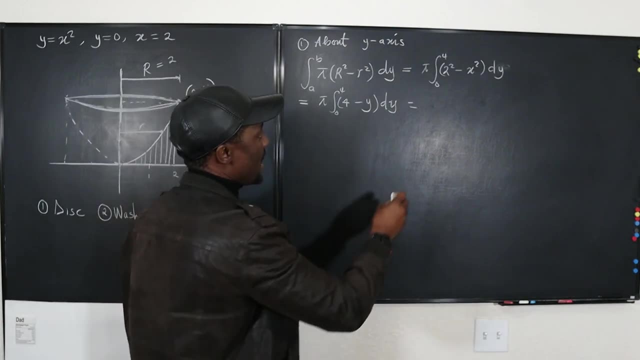 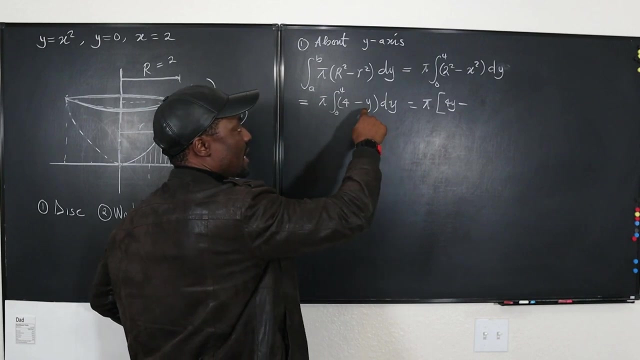 a to b here first from a to b and then we know it's from 0 to 4 0 to 4 and then this is so let's do this integration we've got pi times the integral of 4 is going to be 4y minus the 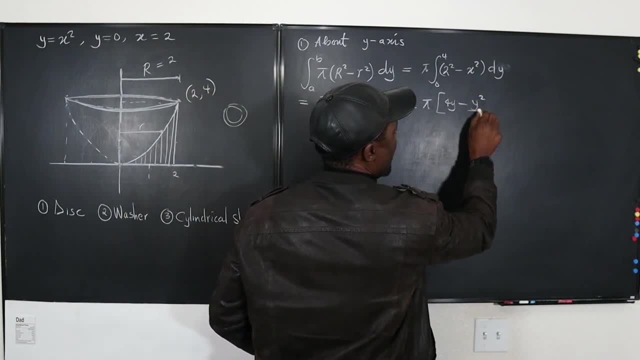 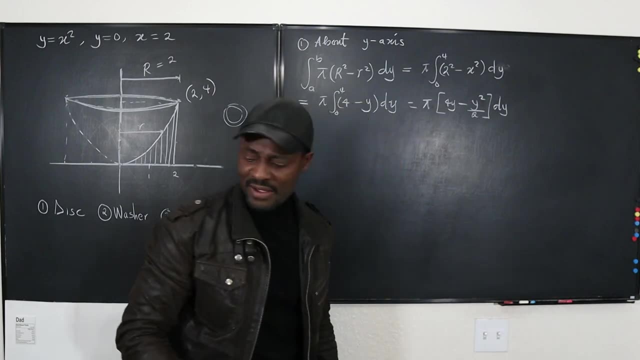 integral of y is going to be y squared over 2 dy oh no more dy just got this 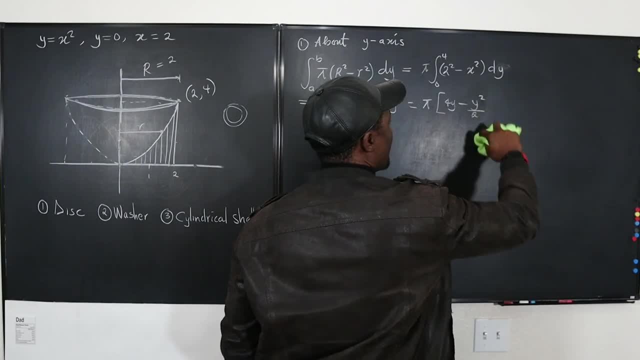 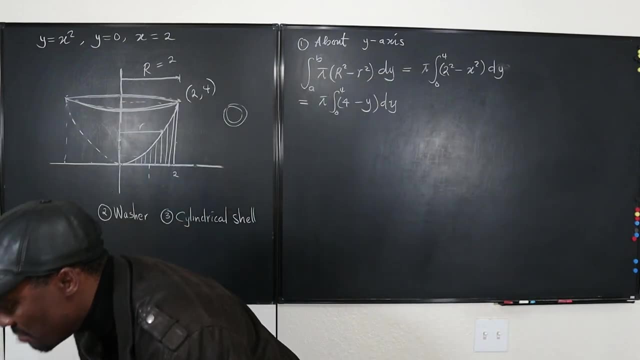 right this has to be muted why are you making sound mute mute mute okay 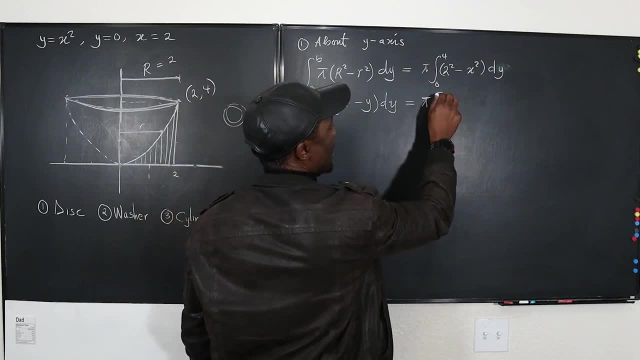 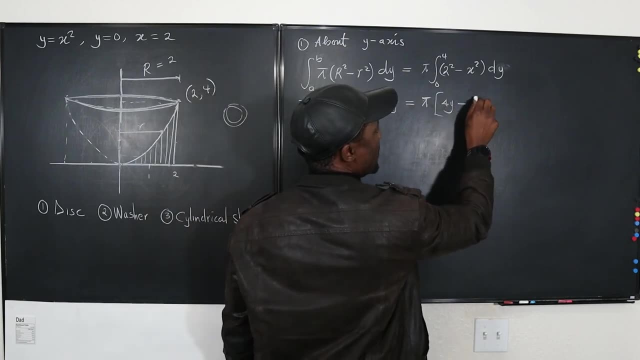 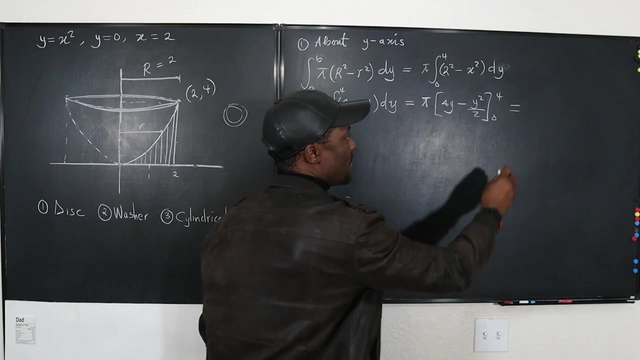 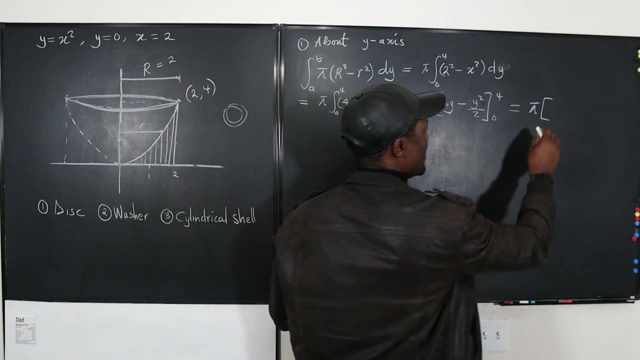 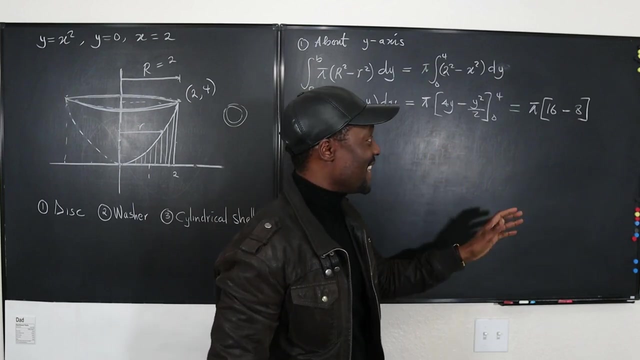 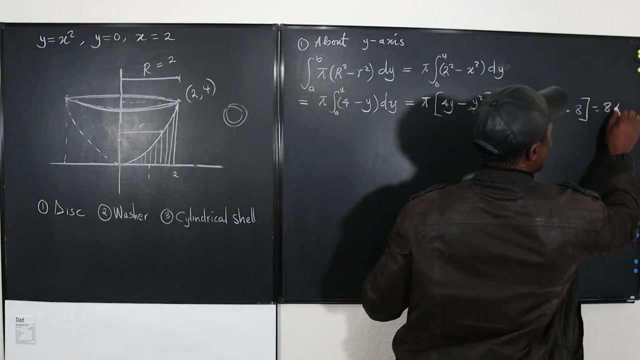 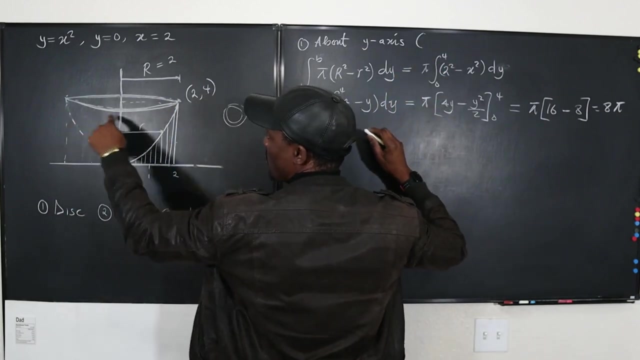 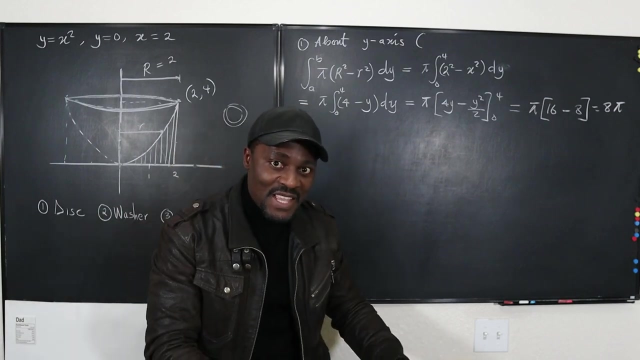 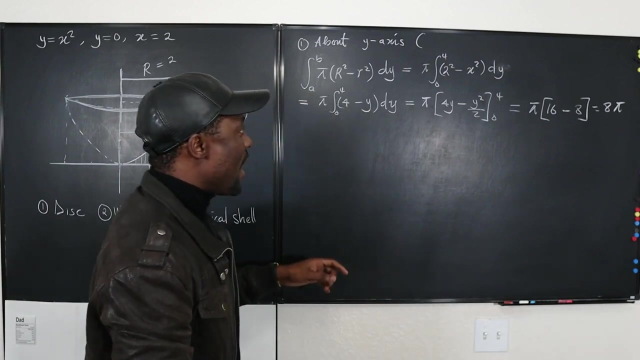 so we take the integral we're going to have pi times this is going to be was the integral of 4 that's 4y was the integral of y that's going to be y squared over 2 evaluated from 0 to 4. okay now if we do this this is going to be pi times well this is 4 times 4 minus 0 so that's going to be 16 minus if we square 4 it's going to be 16. 16 divided by 2 is going to be 8. remember i'm ignoring the 0 because each of if you put 0 in either case you're going to get 0 so i'm not thinking about it so what is 16 minus 8 that gives us 8 and times 5 that gives us 8 pi okay so this is what you get if you use the washer method remember we just use the washer method because this is a washer like i explained because there are two different radii that's how you know it's a washer the inside is closer to this axis of rotation than the outside then you know it's a washer okay now what if i don't want to use the washer method i want to use the washer method instead of the washer method 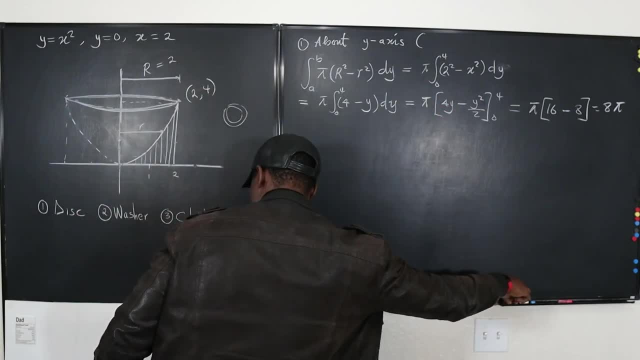 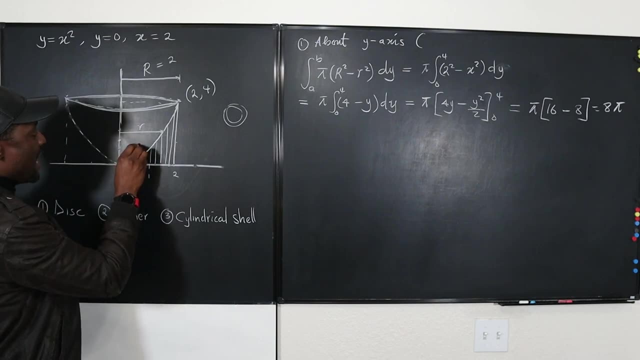 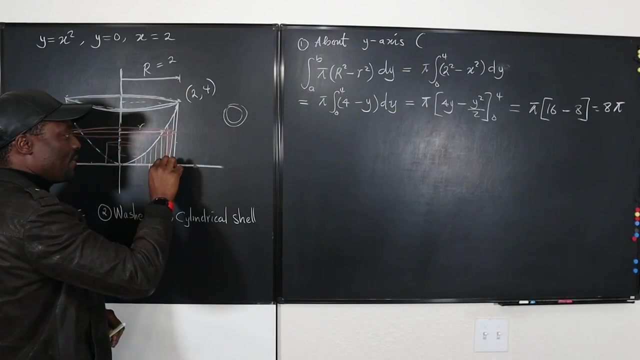 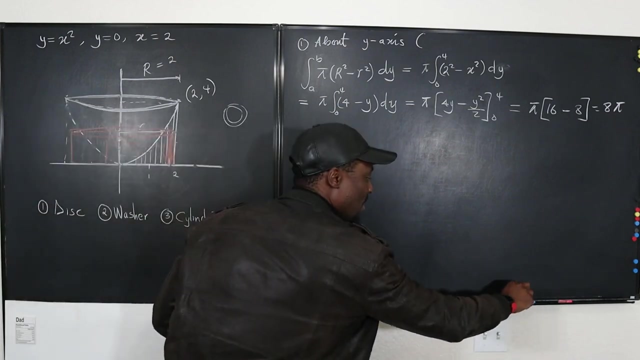 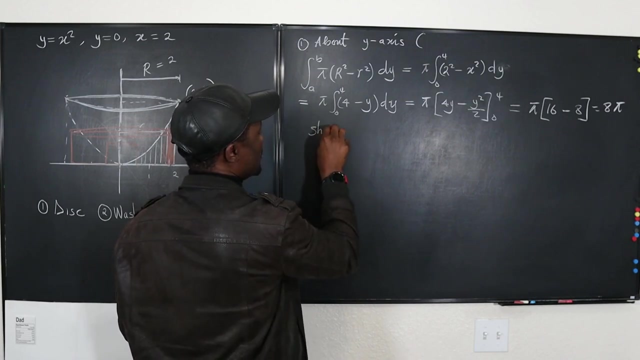 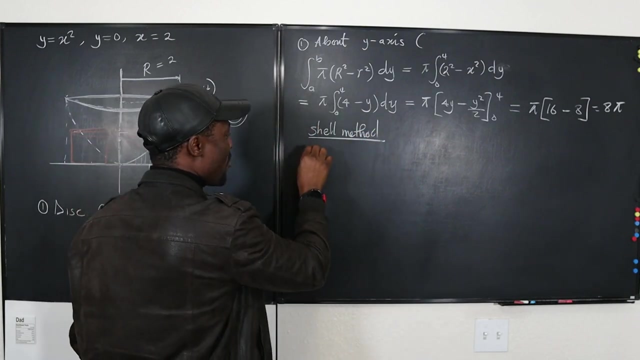 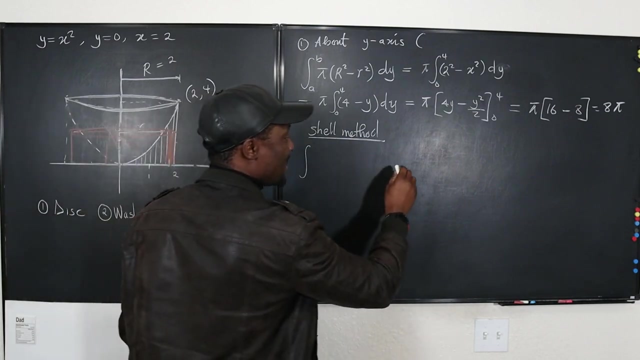 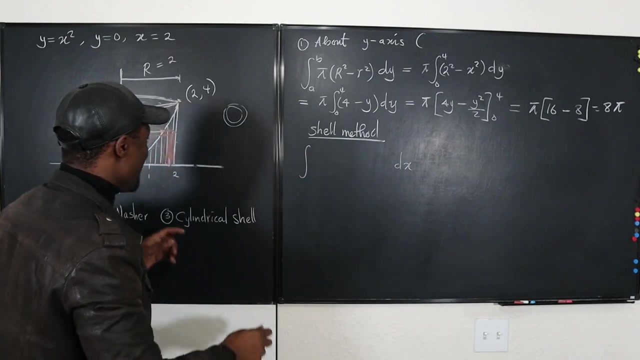 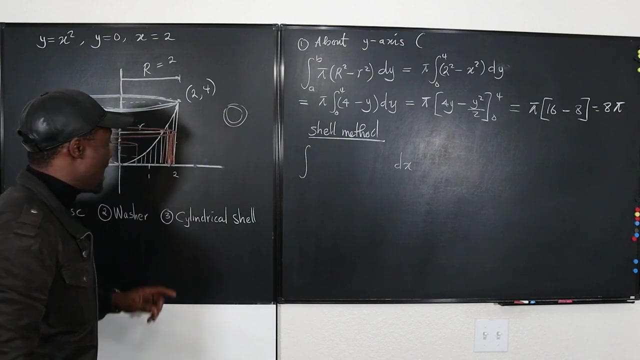 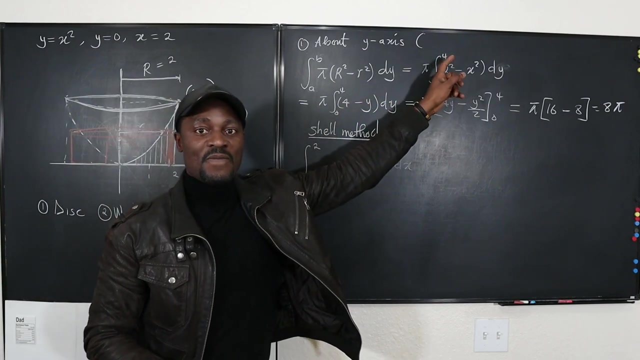 i want to put a cylinder right in here so let's say my plan is or the instruction is don't use the washer method put a cylindrical shell so we're going to imagine that we have a cylinder here okay just imagine you have a cylinder that stretches out so this is not the best cylinder the cylinder has to be something in here it spreads out to this okay like that so at every point you're going to have a cylinder in here and the cylinder will adjust itself and the thickness of the cylinder look it's important for you to know what the thickness of the cylinder is it is getting thicker along the x-axis so this is what i usually tell myself i am going to do a setup so let's still do the shell method shell method okay so what i'm going to do for my setup is from the start i look at what the cylinder looks like it is getting thicker along the x-axis so my integration has to be dx that helps me a lot because because it is getting thicker along the x-axis the next thing i'm going to do is to fix what my bounds of integration they're basically the beginning of the area you're rotating to the ending of the area you're rotating always just look at the area you're rotating from zero to two so i'm going to write zero to two you can see it's different this is zero to four okay so it's from zero to two i'm rotating i'm rotating and that's it what do you need to put in here 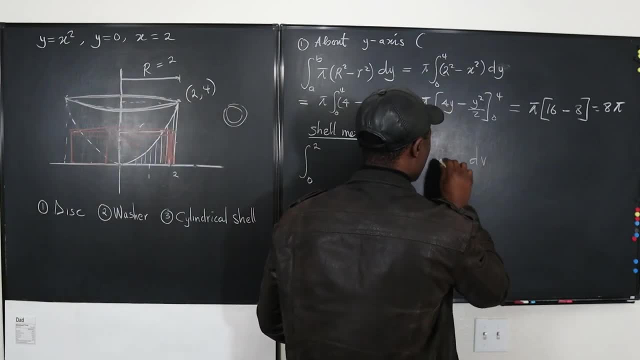 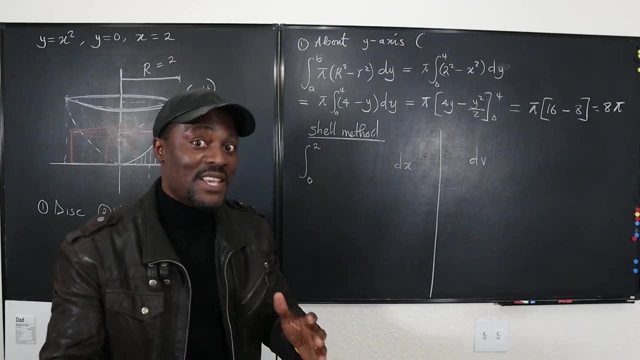 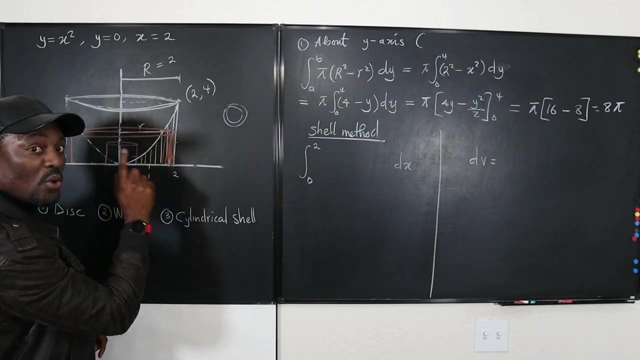 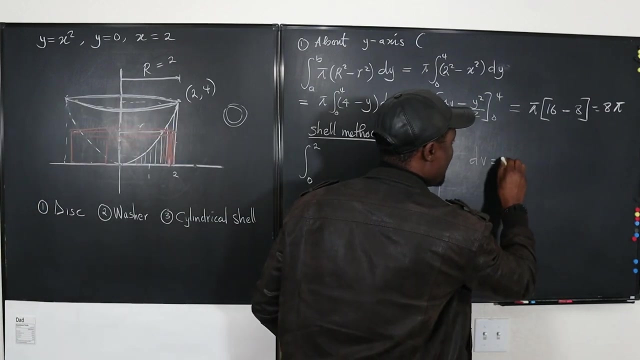 now let's talk about that i usually like calling it dv okay so dv is what i'm going to put in here because when you integrate dv you're going to get v okay what is dv dv is basically the circumference of the cylinder multiplied by the height of the cylinder integrated along the thickness so it is usually the circumference 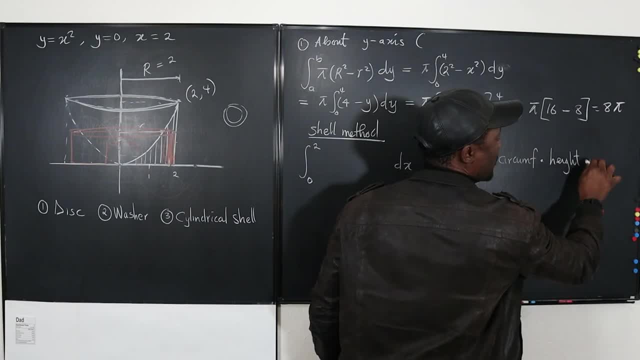 multiplied by height multiplied by the thickness 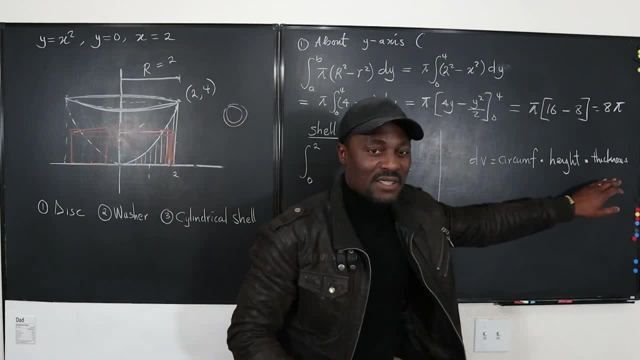 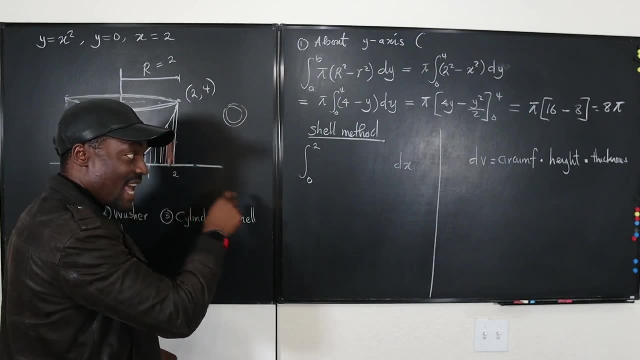 so what is the circumference of this what is the height what is the thickness we already identified the thickness that's delta x oh man that's dx rather so thickness is dx i started with that so that's done 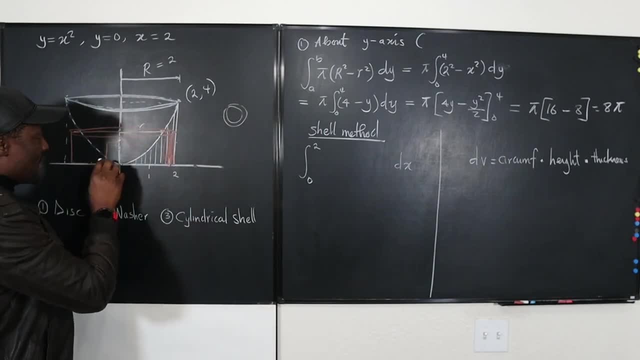 height of this cylinder now at every point the height of this cylinder is determined by this function so this cylinder that I put here cannot even exist because it has to be as high just as high as this function so this would be the cylinder at this point at this point this is gonna be the cylinder you see all the shapes I'm having it's getting rough okay but that's the cylinder you get this is the cylinder at this height so the height of the cylinder is basically the height of this function which is basically what you can 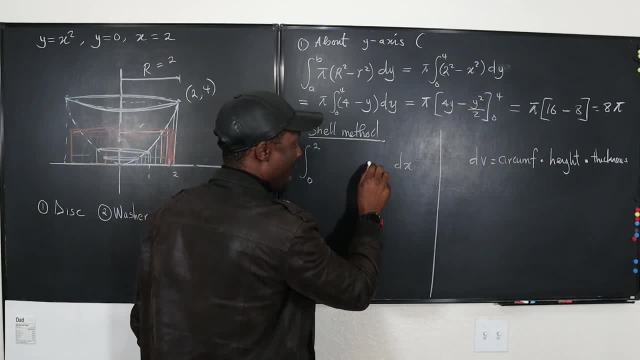 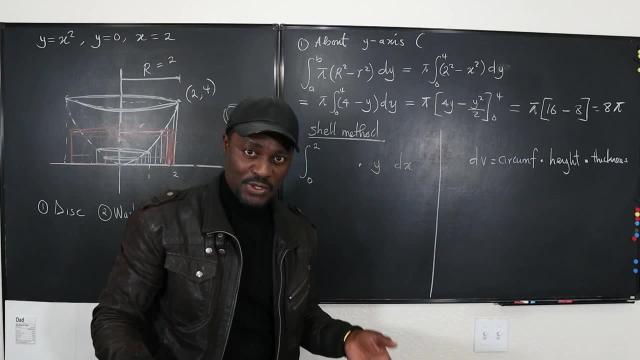 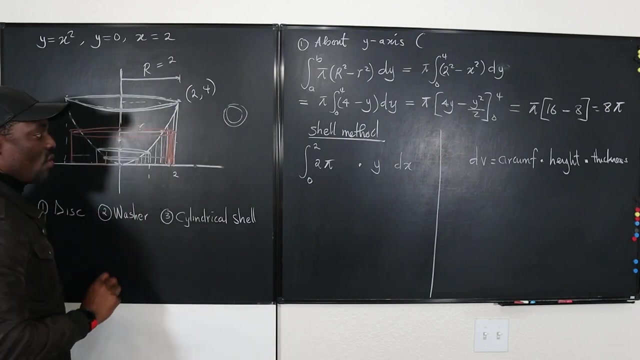 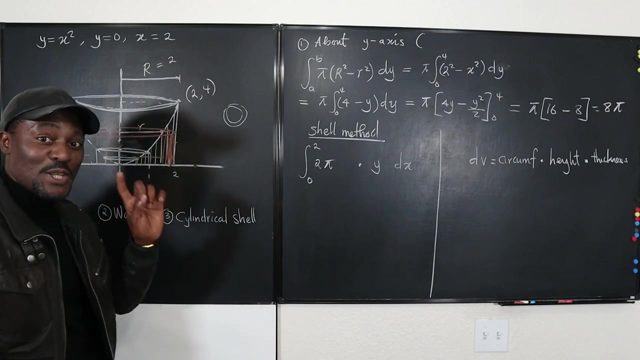 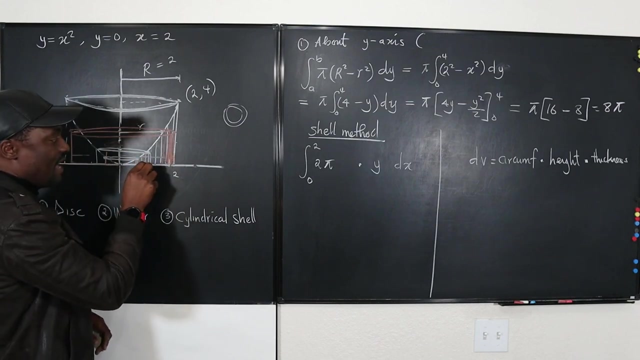 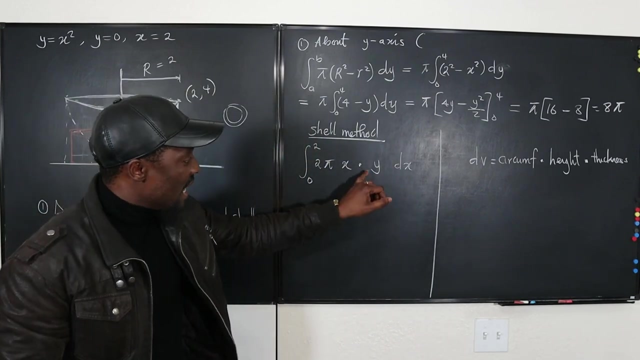 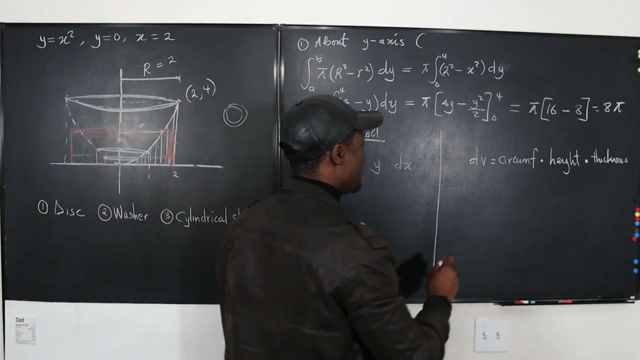 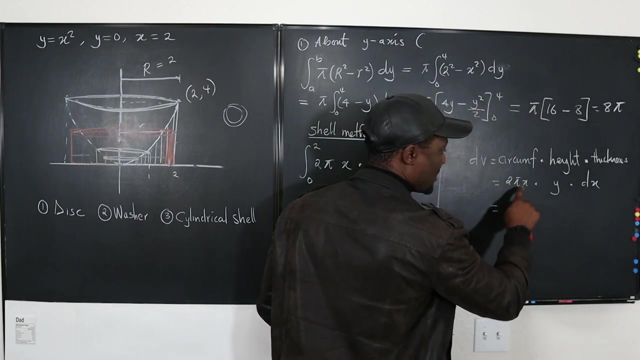 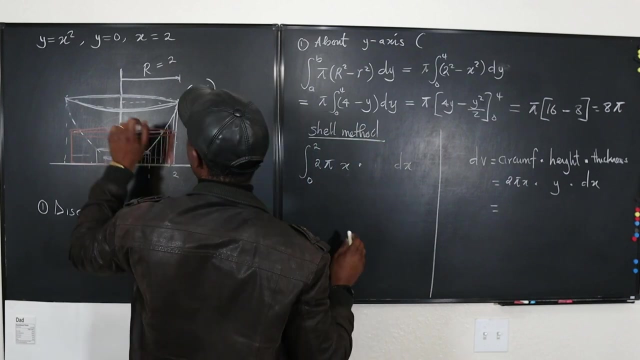 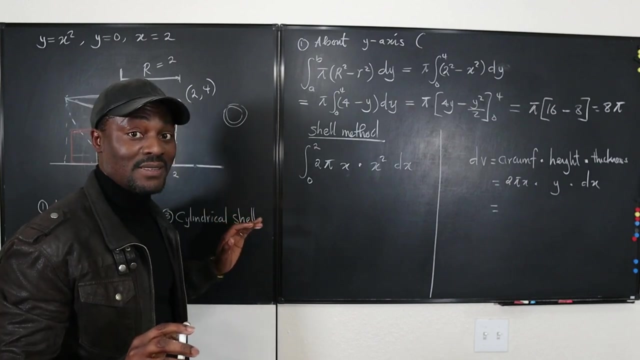 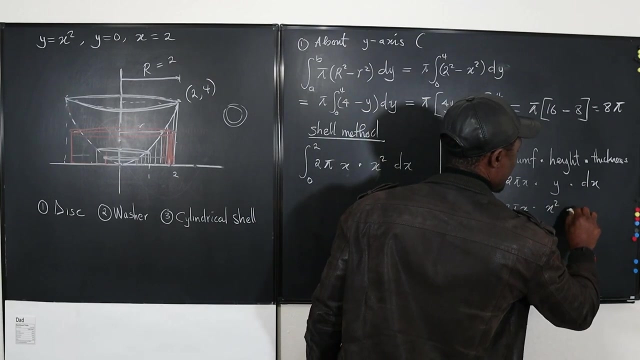 read off of the y-axis so the height of the cylinder is y so now what about the circumference formula for circumference of a cylinder is a circle it's 2 pi R 2 pi now what is the radius of this what is the radius of any cylinder okay basically it's 2 pi R the R is going in this direction okay so remember it's a cylinder we're not talking about a disc or a washer it's a cylinder so the cylinder has only one radius okay and it's any point the cylinder is if it's here that's your radius and that's the value of X you're gonna get okay so it's gonna be just X beautiful the only thing that is not okay is the Y because we're integrating with respect to the y-axis so that's the only thing that is not okay is the y because we're integrating with respect to X so what we have here is two PI X times y times DX okay what this add has to be changed so because I cannot put X I mean I can't put I can I'll put y here rather what did we say why was y is x squared so I think that's the only thing I need to change okay and with that we can say this is 2 PI X times X squared dx okay let's get our y-axis we got to read that 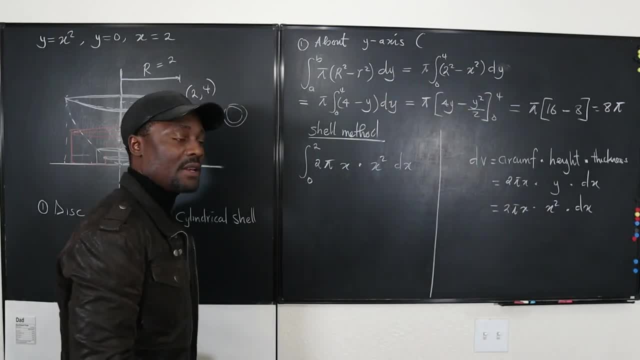 dx. And that's what I'm going to bring in here and integrate. So this is the same thing. Let's clean this up. This is 2 pi x cubed dx. So I'm going to clean this up and put the correct thing. 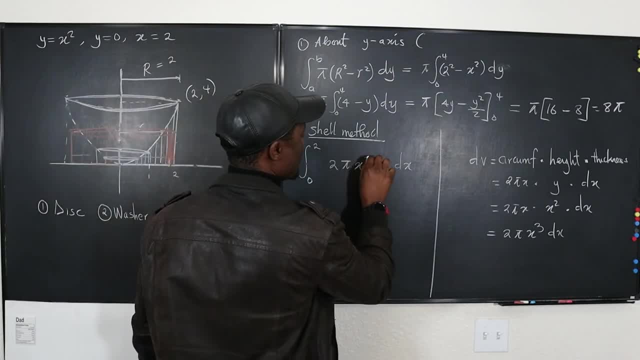 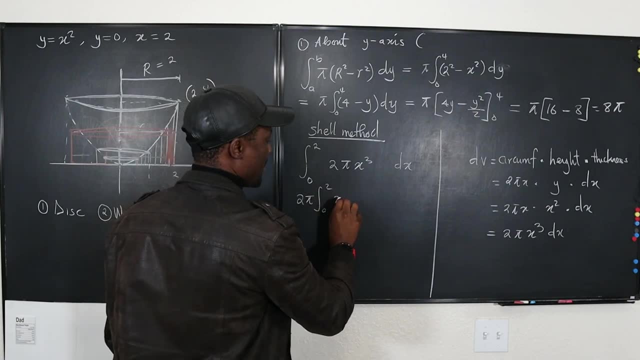 So this is going to be 2 pi x cubed. Now, let's integrate. This is going to be 2 pi integral 0 to 2 of x cubed dx, which is equal to 2 pi. 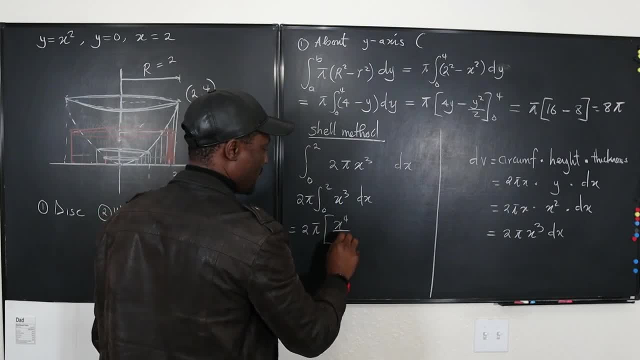 If we integrate this, it's going to be x to the fourth over 4 from 0 to 2. This is going to be 16 sorry, 2 pi. 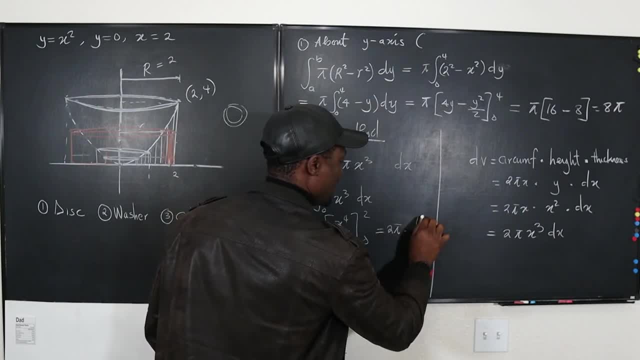 It's going to be 2 pi times 16 over 4, which gives us 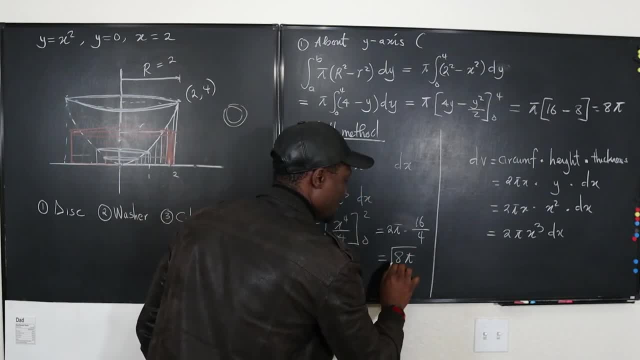 that's 4 8 pi. 8 pi. As you can see, it's the same exact answer we got. 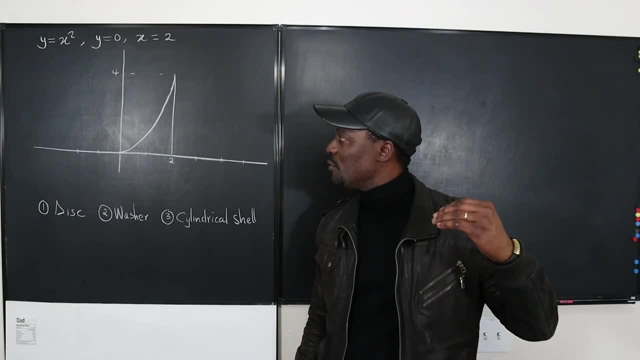 When we solve using for the second part, I am going to rotate instead of rotating it this way. I am going to rotate this way. 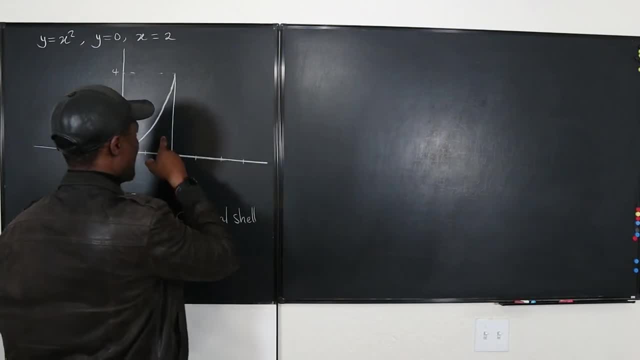 So now look if I rotate this part here because there's no hole. There's not going to be a hole here. This is what it's going to look like. 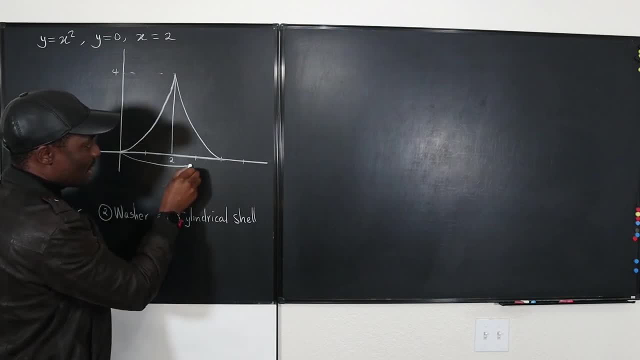 So you see that the rotation is going to look somewhat like this. 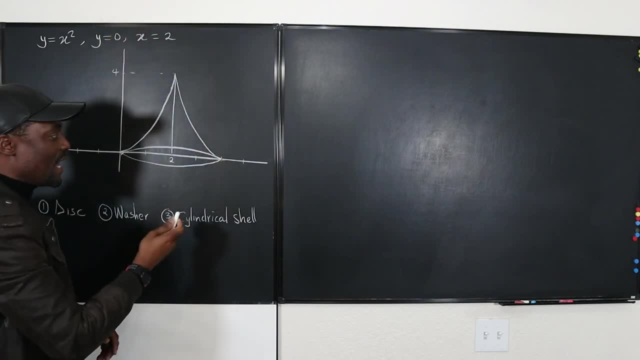 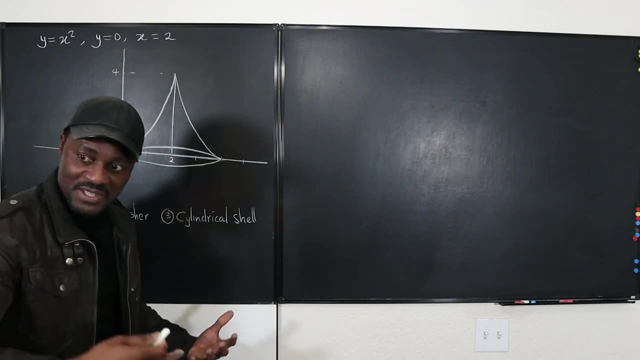 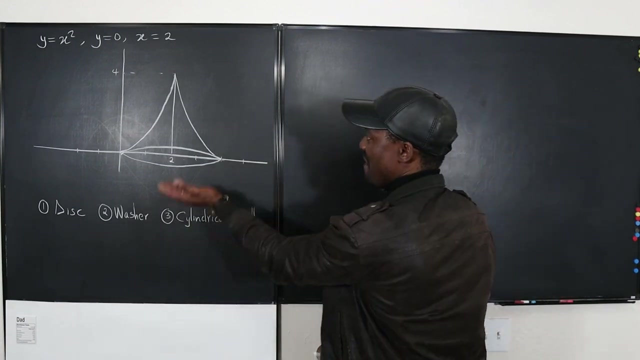 So I'm going to have disks stacked up this way. There is no hole in the middle because this is solid. Unlike the previous time when I rotated that you could put something inside the bowl. And if you could put something inside the bowl, then you have to it has to be a washer, but now everything is solid. 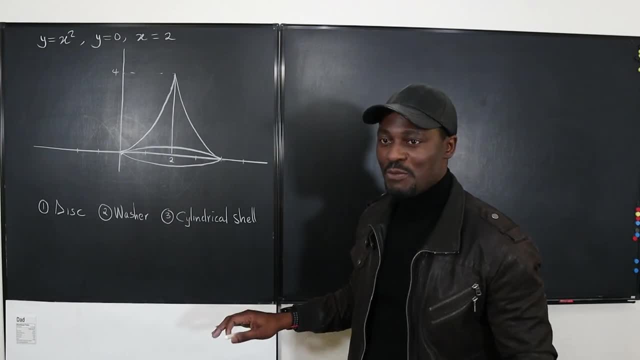 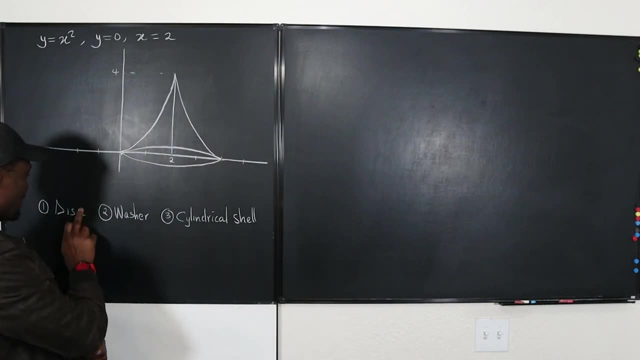 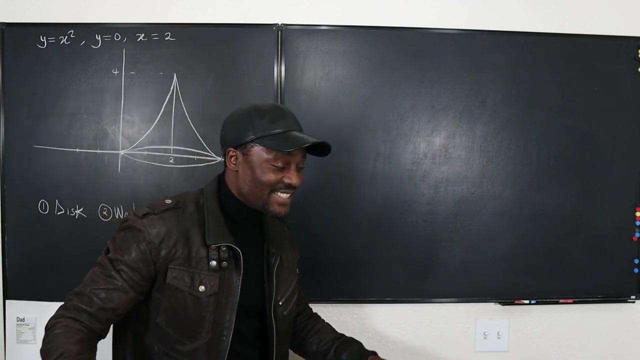 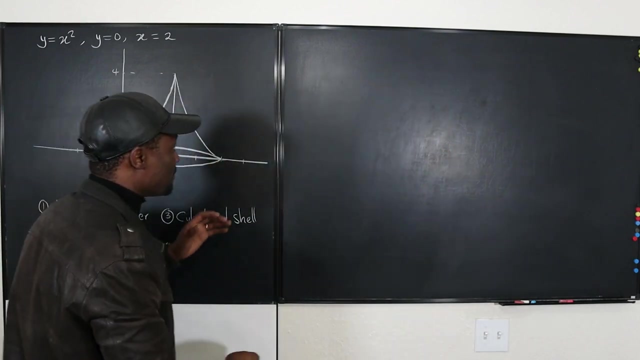 Okay, there is no hole. There's no internal radius. So you notice I just have a bunch of disks stacked up. So we have to solve this using the disk. Well, I spelled my disk this way. I might change it to k. I'm so sorry. If you live in America, disk is D-I-S-C in the British spelling regime. Whatever you call it. Okay, so So you have we're going to use the disk method. 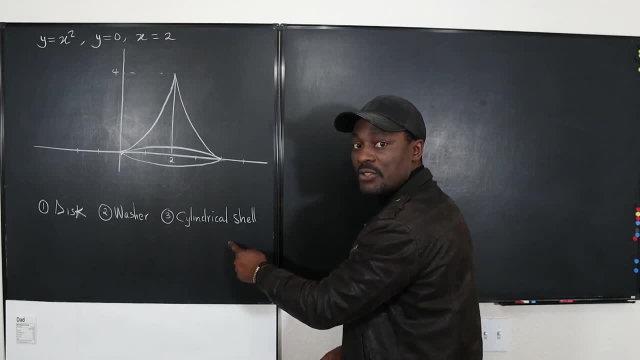 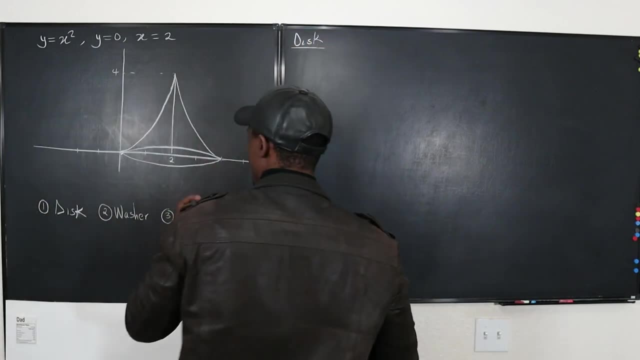 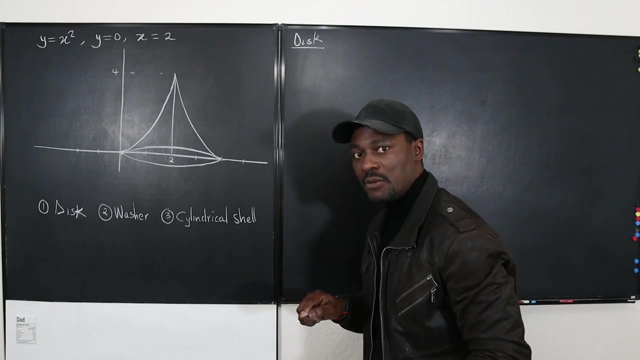 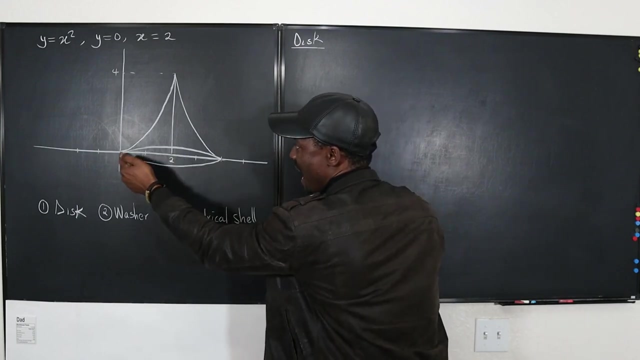 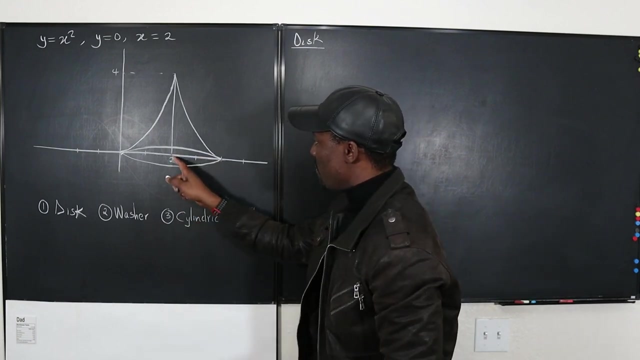 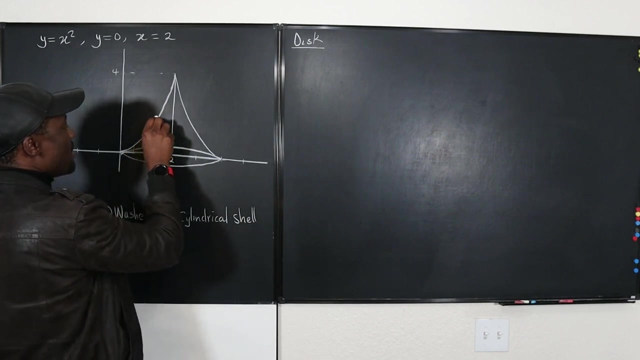 And I'm going to also show you that you could do it using the cylindrical shell method. So let's use the disk method first. So let's do disk. So remember that this is basically area times height. Because the height is not uniform, that's why we integrate. Okay, the height is not uniform. We have to integrate to generate the height. But the disk the area of each face is just 2 pi. Whatever the radius is, you can see the radius is from here to this point and from here to this point. But because this is the real part. So this is where many students get this wrong. This is the only way. 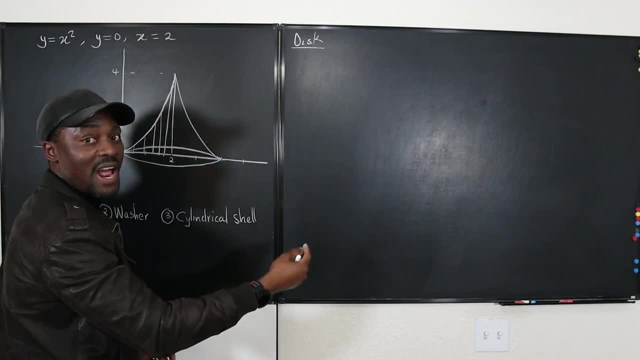 is the original part. This is the part that is generated after rotation. So your focus should 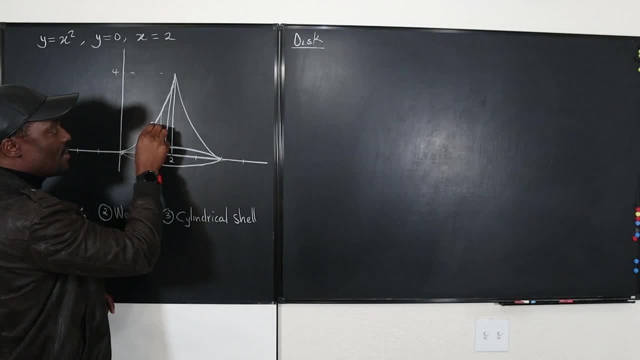 be here. If I want to determine the distance from here to here, what do you think I'm going to do? 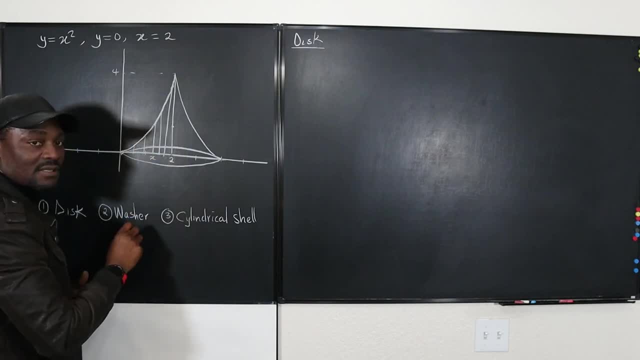 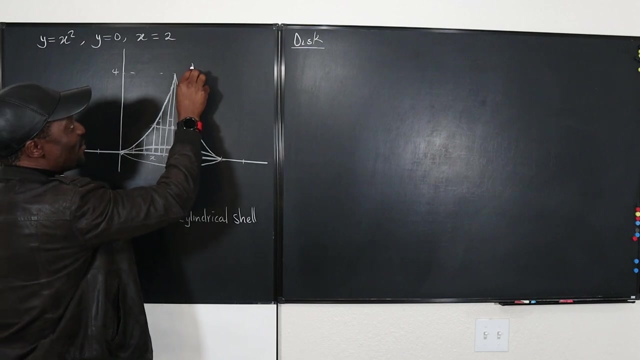 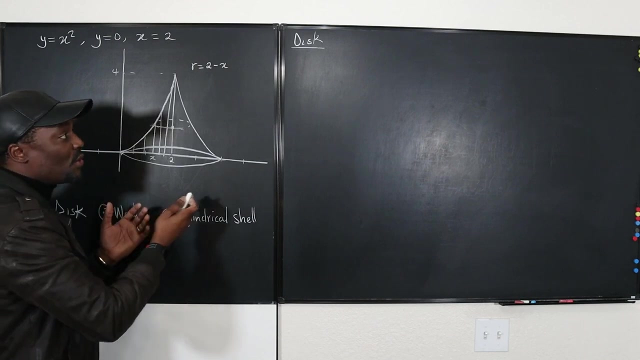 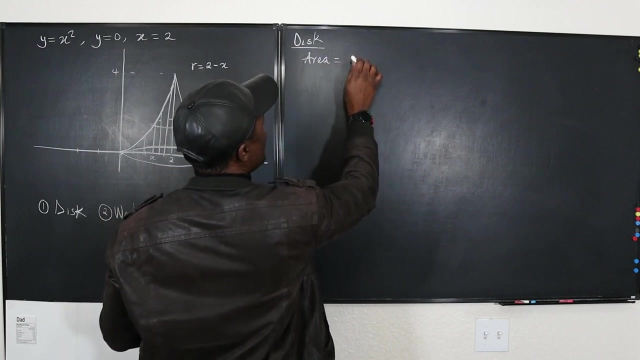 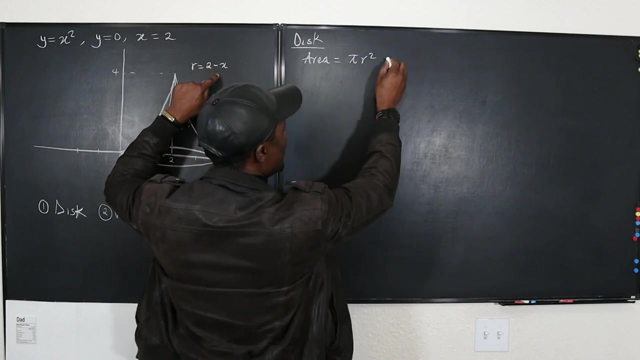 Remember, at every point here down here, you can call this x. x is changing depending on where you are, okay? Whether you're up here or down here, the value of x is changing. But the radius of each of the disc at each point, the radius of every disc that you're going to cut is the distance from here to here. The distance from here to here, which is 2 minus x. That's your radius. So the radius, remember that, your radius equals 2 minus x for this disc to work, okay? So here, we're going to go here and say that the area... is equal to... Remember, it is pi r squared. Pi r squared. Which is the same thing, since the radius is 2 minus x. That's going to be pi times 2 minus x squared. Well, we'll have to distribute this. 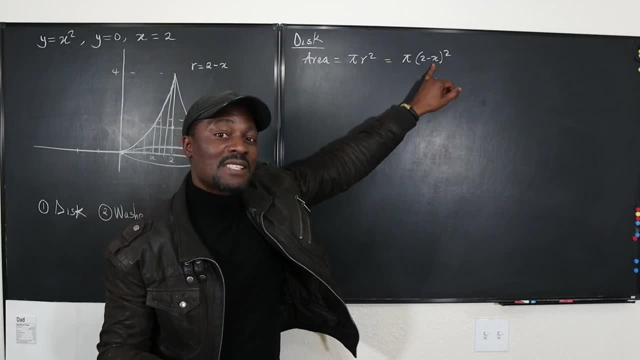 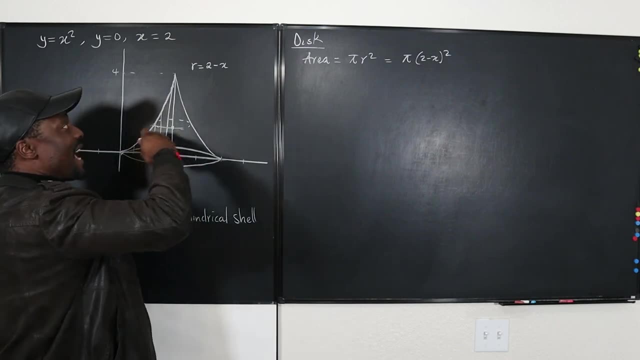 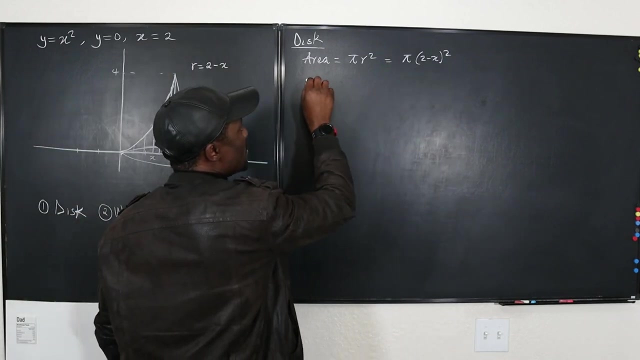 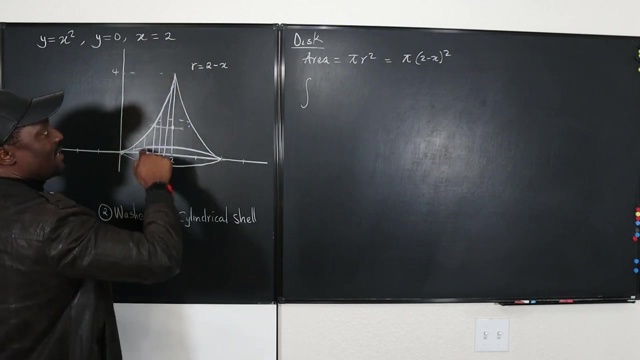 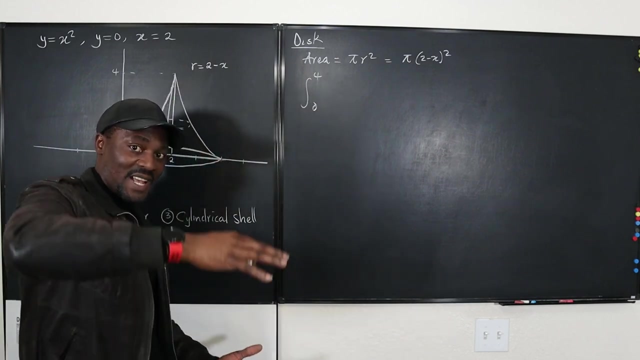 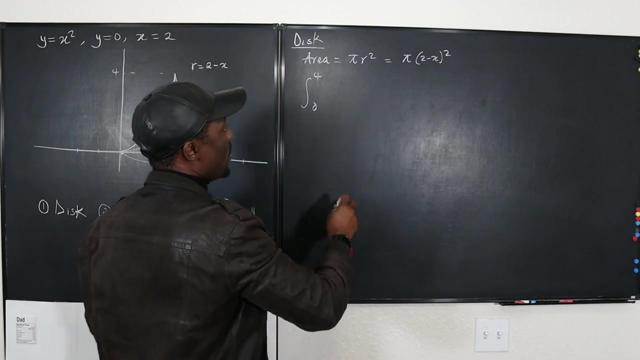 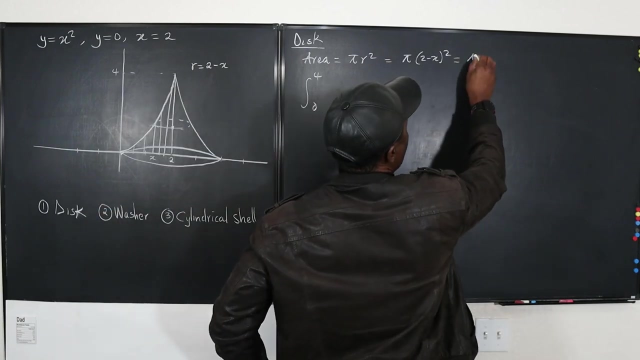 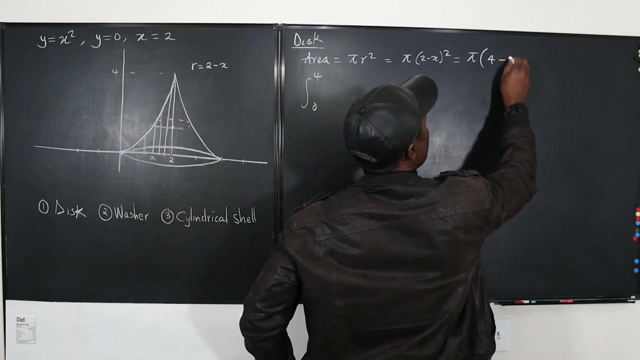 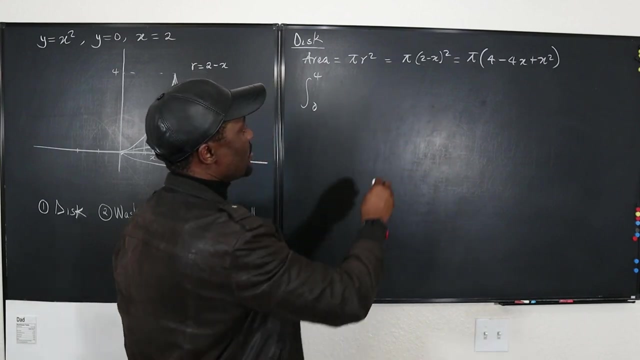 Why? Because we can't leave our work in terms of x, because I already know that our d... our differentiation of the thickness of the disc, they stack up along the y-axis, so it has to to be dy. So I have to come here and say whatever I do will be the integral from the beginning to the ending. This is the beginning of our stacking from zero to four. Okay? Thickness. Remember you always go along with the thickness of the disks. Now, so zero to four of the area. Okay? So what is the area 2 pi r squared which is gonna be pi...sorry sorry pi r squared? And if you FOIL this out you're gonna end up with 4 minus 4x plus x squared. Okay. Now, we can all put that, remember it's gonna be dy. So this is gonna be, let's put the pi outside here. So we're gonna have 4x. 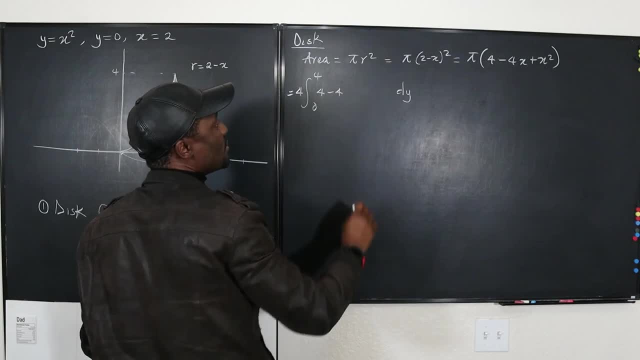 minus 4 times x. What is x? We can replace x squared easily like we did in the previous one 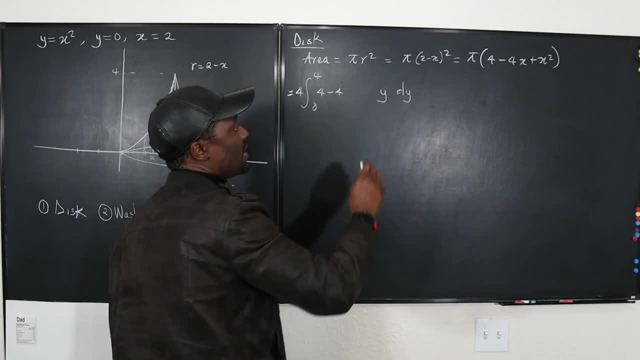 with y. So we can put y here. But what will this be? x is the square root of y. So from here, 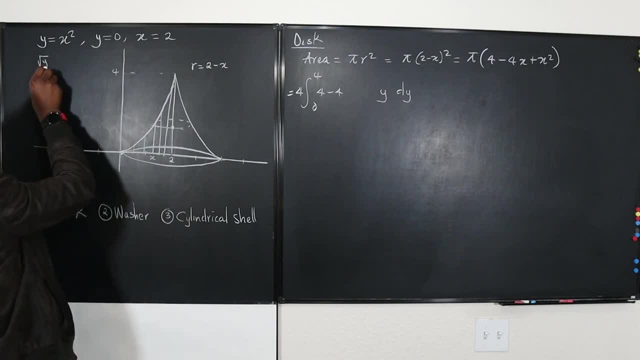 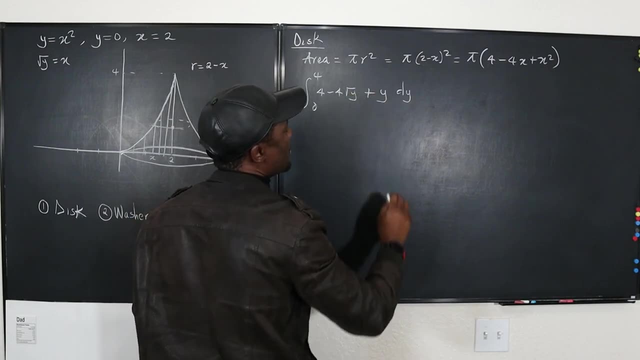 since we know, we can say that the square root of y is equal to x. So we can write the square root of y, okay? And then here we have plus. And this is the function, this is pi, this is the function 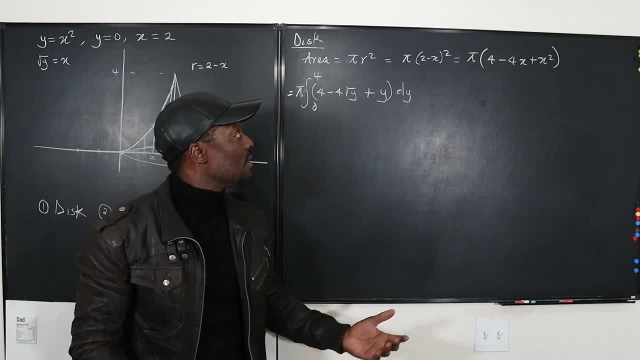 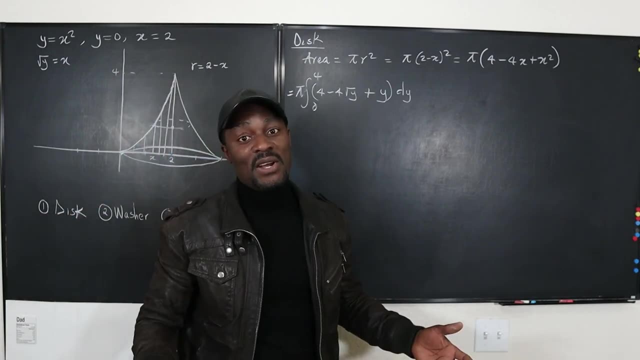 you will have to integrate to get the value, the volume that we're looking for using the disc method. So the disc method is not always that straightforward. It depends on where you rotate, 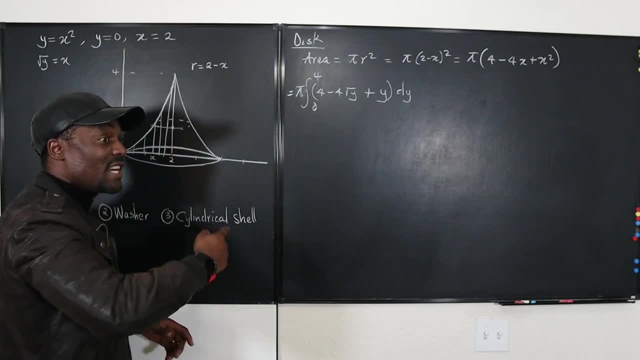 okay? Especially if you rotate along a line that is not zero, your radius will be that line minus something. 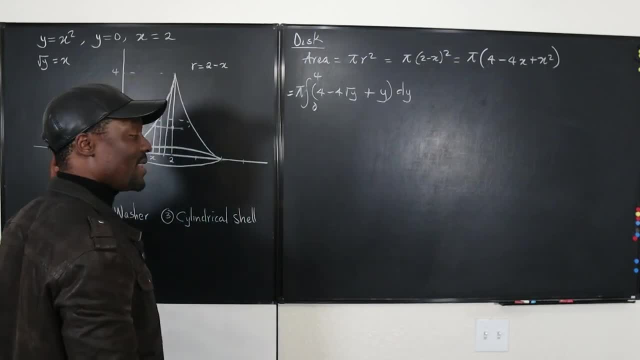 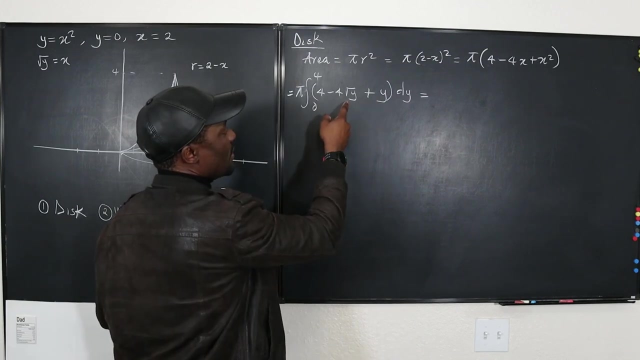 Remember that. Or that line plus something, depending on whether the line is here or the line is here, okay? If the original is to the left, it's going to be a minus. If the original is to the right, it's going to be reversed. x minus whatever that is. It may be difficult to 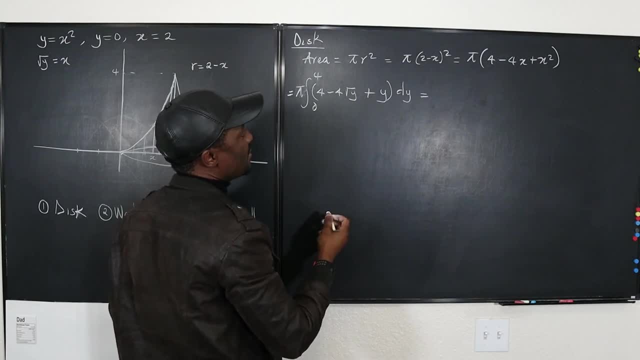 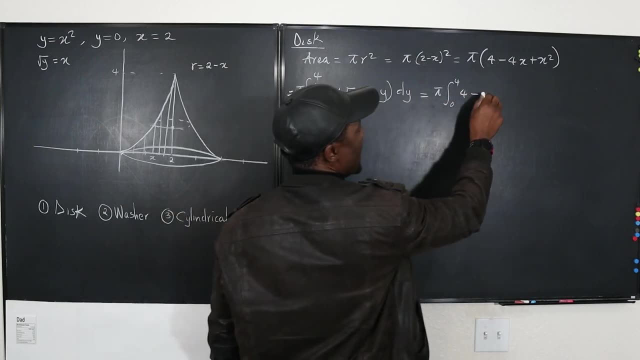 integrate this, or impossible actually. I have to write this as an exponent. So this is the, this is equal to pi integral zero to four of four minus, I write this as an exponent, that's going to be four y to the... 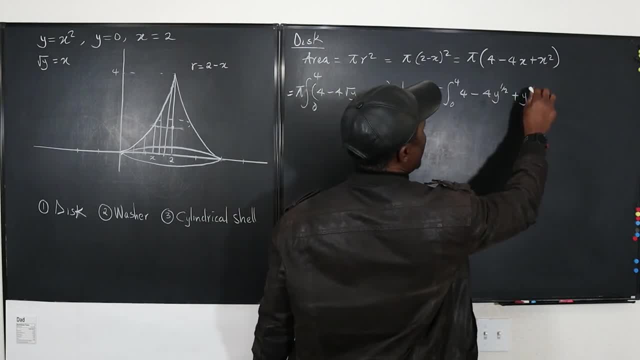 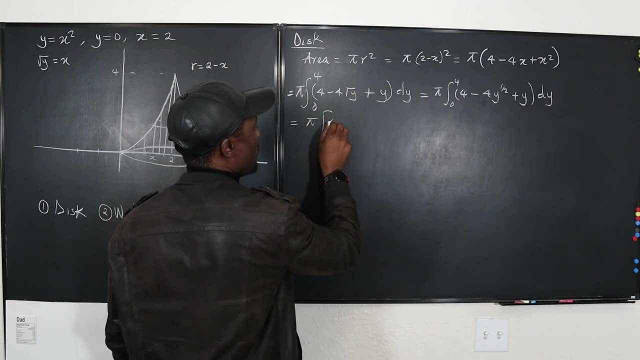 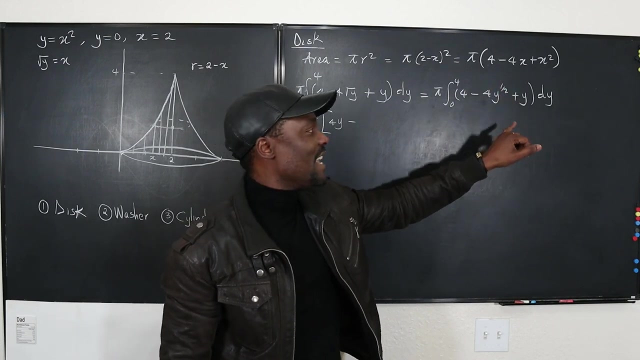 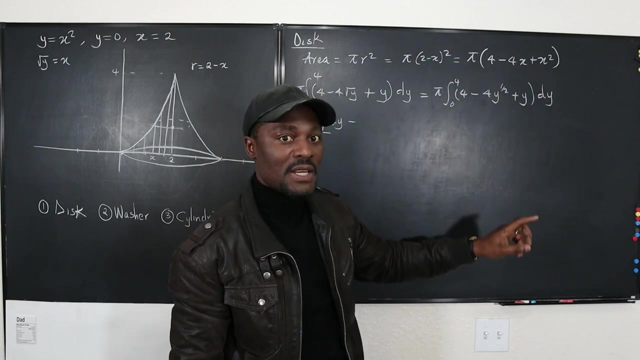 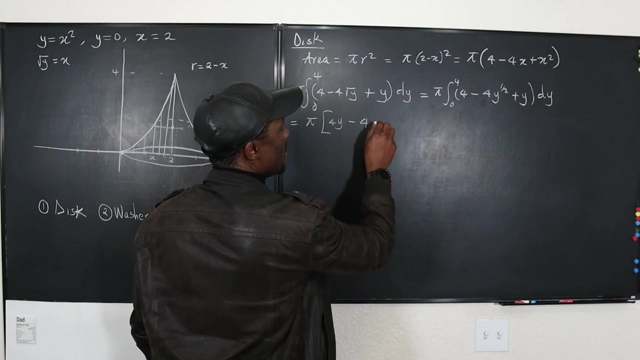 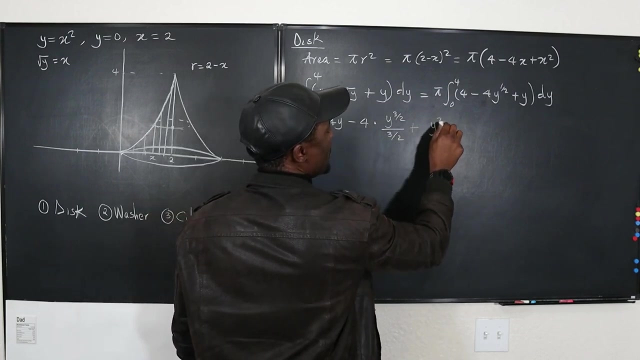 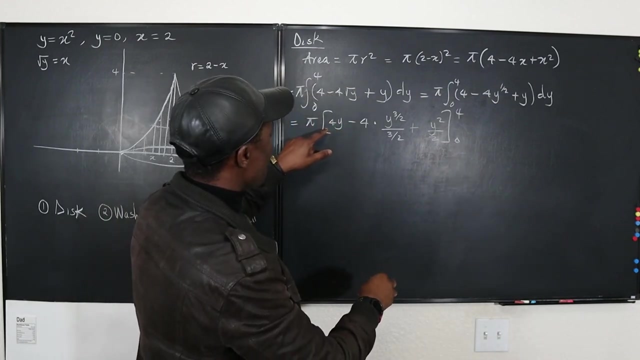 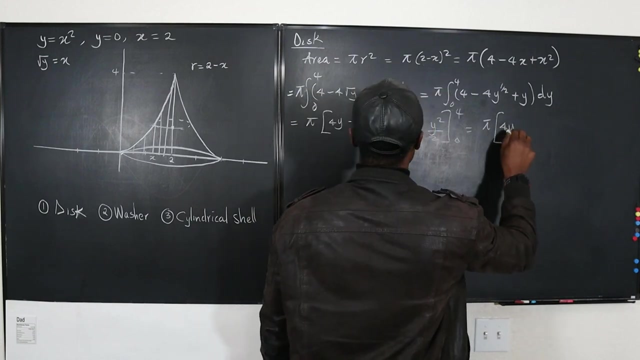 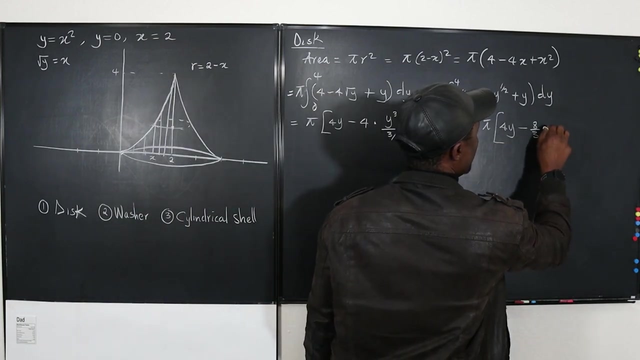 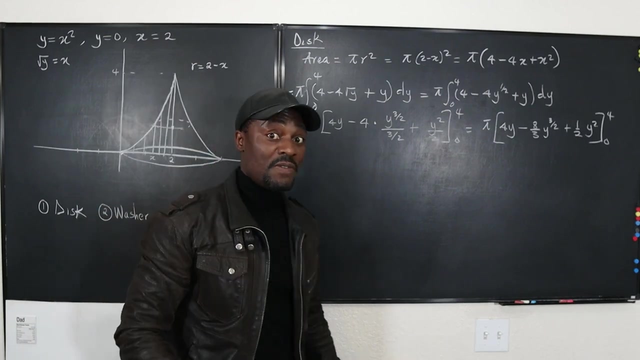 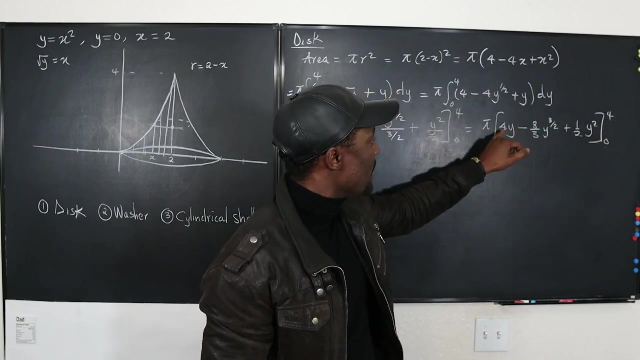 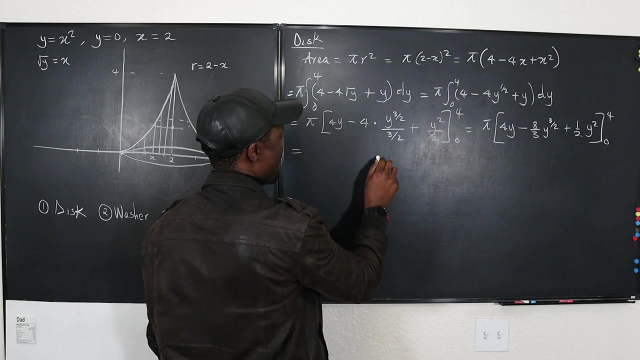 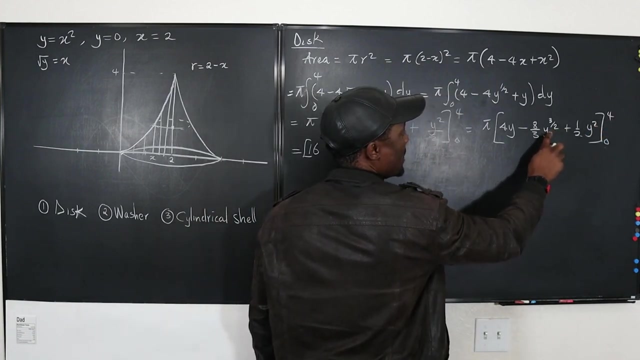 So one half, and this is plus y, and then I am going to do dy. So this is equal to pi times, if we take the integral, this is going to be four y minus, if we integrate this, remember what I've shown in other videos, to integrate any fraction is easy. Just say any function, any variable with a fraction exponent, just add the two together. Three plus one gives you, sorry, two plus one gives you three, and then you divide by two. So it's three over two. So it's three over two. So it's going to be minus four times y to the three halves over three halves, okay? Plus, this is going to be y squared over two, evaluated from zero to four, okay? Now, because, let's clean this up first. So this is going to be pi times, this integral is going to be four y, and this is going to be, if you flip this, it's going to be negative eight over three. So that's minus eight y to the three halves, and that's going to be plus one half of y squared, okay? Evaluated from zero to four. Now, I'm going to do a final evaluation, because each term contains y, the zero is not going to count for me. So I'm just going to focus on the four. Now, four times four is 16. So this is going to be equal to 16. So there's pi. I'm going to put pi at the end. So here's pi, and I'm going to put pi here. I have 16. Now, I put four here. The square root of four is two. Two times three is, so the third power is eight. So that's going to be eight times eight. That's minus 64 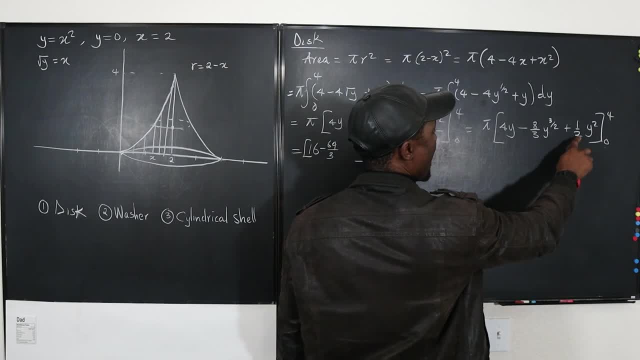 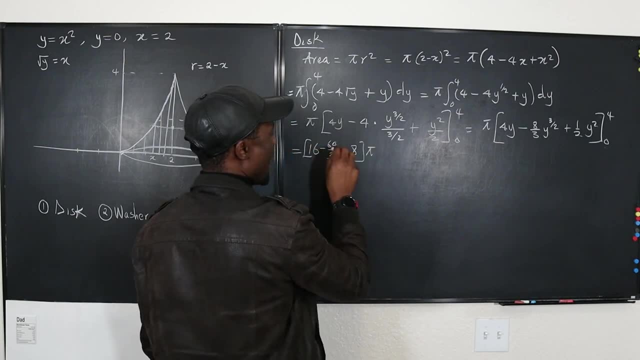 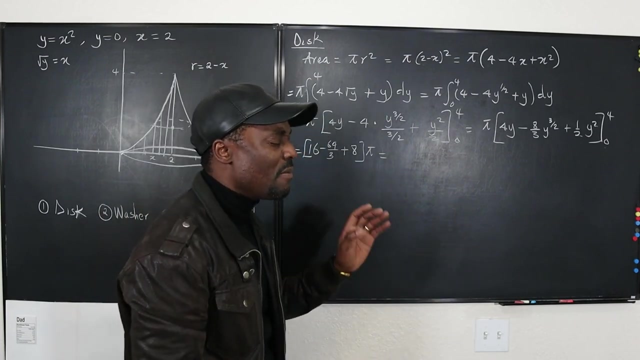 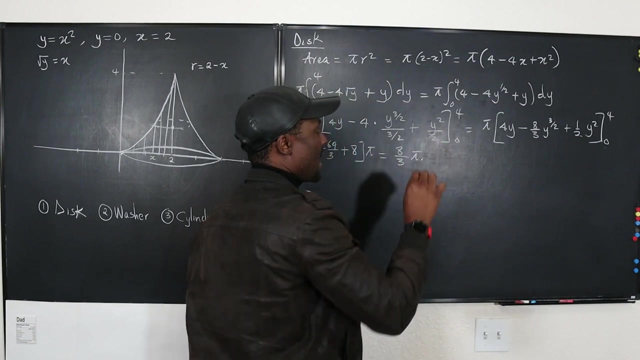 over three, okay? And then I have 16 is four squared divided by two. That's going to be eight plus eight. So what I have basically is 24 minus 64 over three. That's going to be 72 minus 64. That's going to be eight. Oh, it's eight over three pi. And that's the area that we're 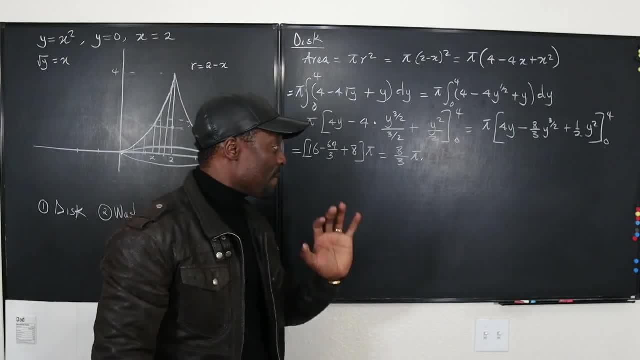 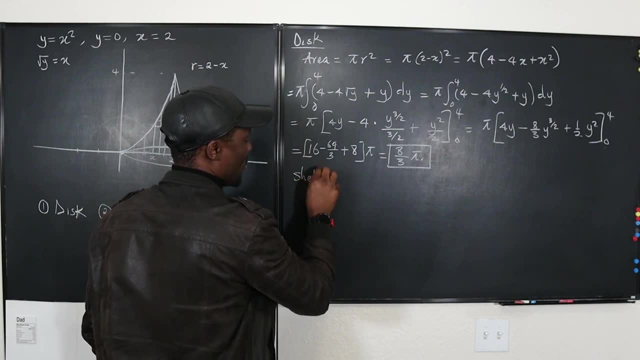 looking for. Okay. Now, we're going to do the shell method, okay? Let's see if the space will take it. 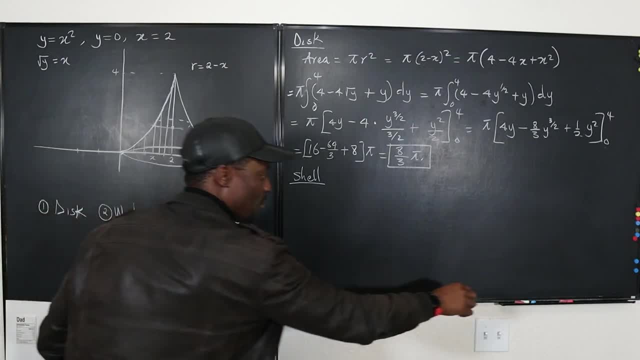 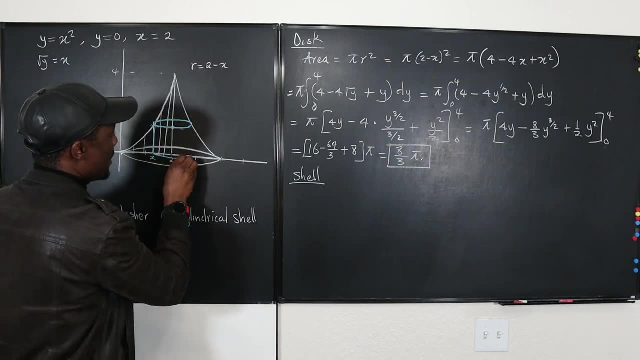 Let's do the explanation here. So look at what I'm going to do. I'm going to insert a cylinder here, okay? Let's say this. This is a cylinder, okay? Like I said, the cylindrical method always works. It's a universal 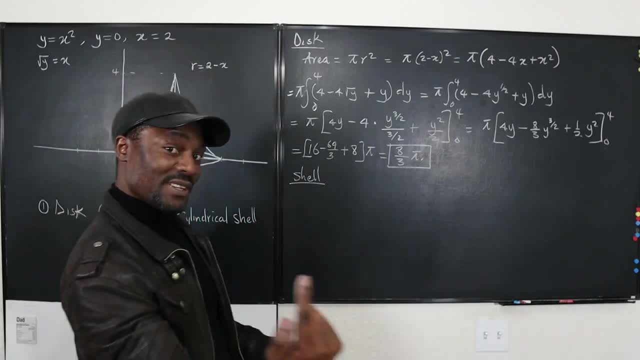 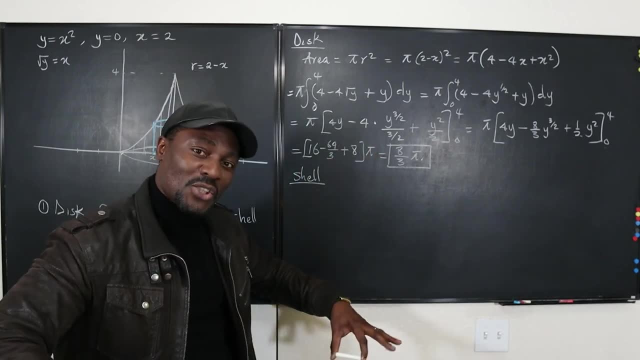 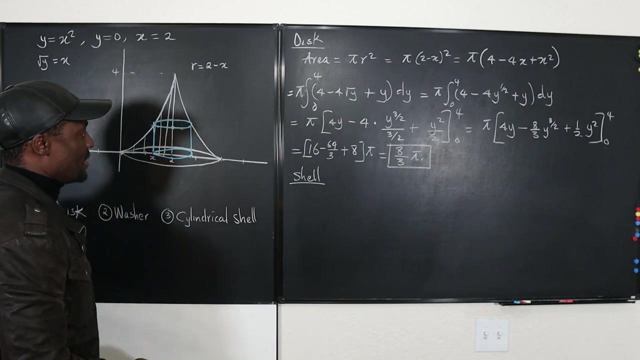 method, okay? Because every time you go round, you are creating a cylinder. It may not be perfect, but it's a bunch of cylinders with different radii and thicknesses that you're working with, okay? So look at this. At any point, the radius of this cylinder, let's say this, is the distance from the center to this point, right? This is the part that we're dealing with. So the radius of this cylinder is basically anything. Remember the cylinder 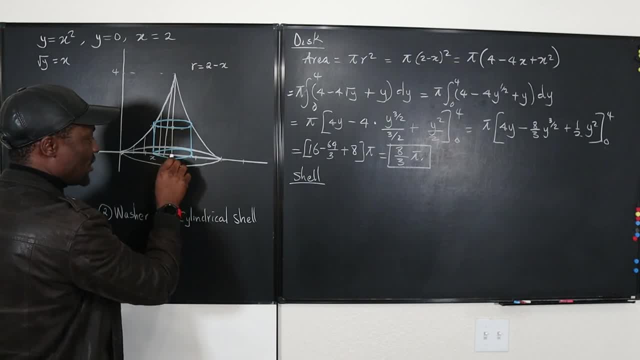 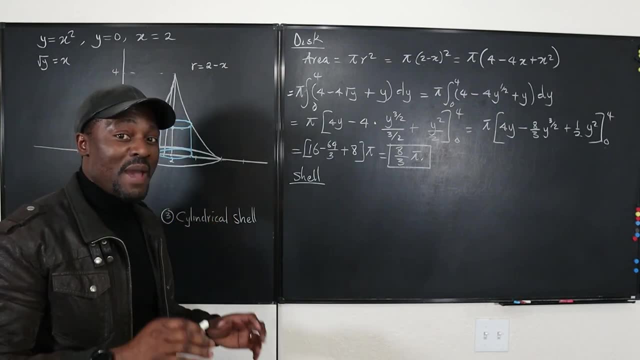 will thicken out, okay? So the radius of the cylinder is just x and that's the first and the most important thing. You're going to integrate with respect to x. 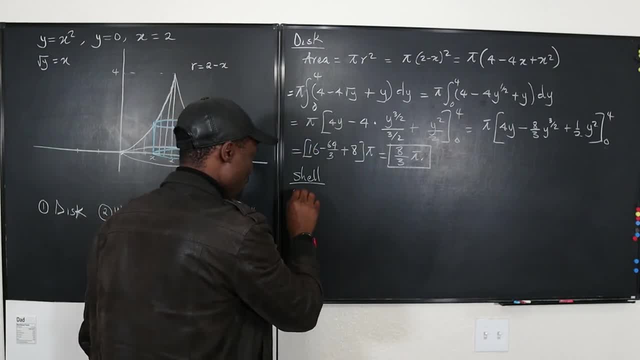 So I'm going to say finally, when we do our integration, we're going to be doing the integral of this. of this original portion. 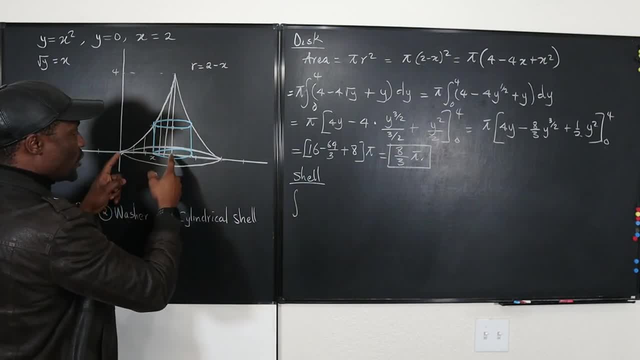 That's how you do for whenever you do the shell method, just look at the original portion is from zero to two. 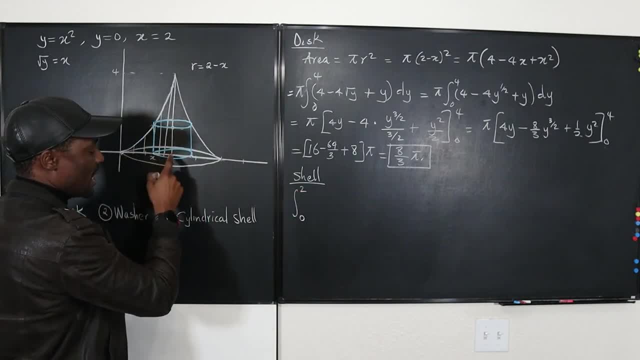 So it's from zero to two of the original portion and you're gonna be integrating doing DX. 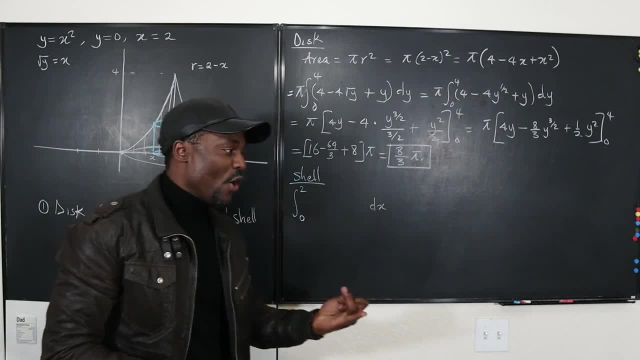 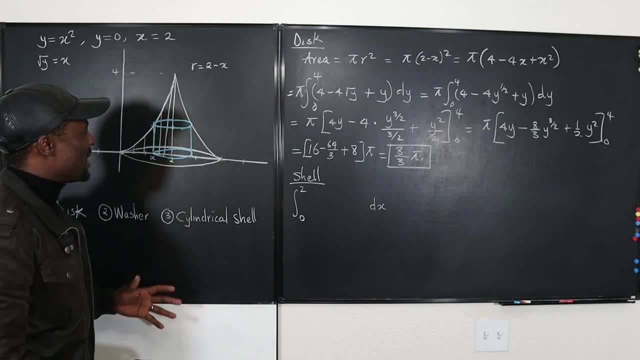 Your business is to find what the area of the circumference rather of the cylinder will be and what the height of the cylinder will be. 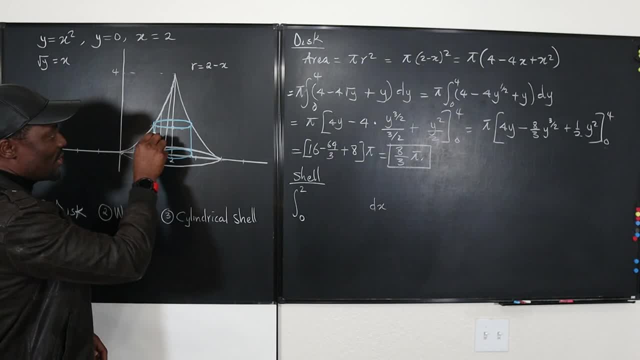 The height of the cylinder is not a problem because the cylinder, you take the height just based on whatever this function is at this point. So it's just Y. That's the cylinder. Whatever you get here as the height is Y. So we know that the height of this cylinder is gonna be Y. 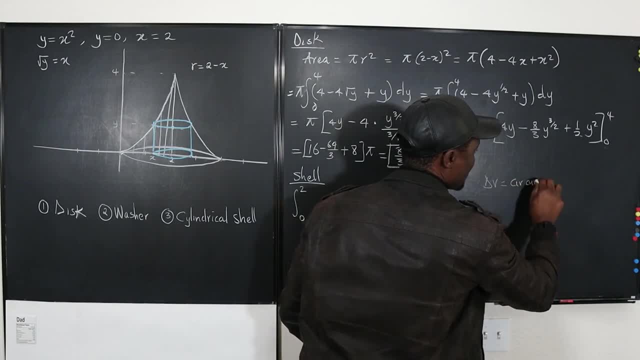 So let's do the V here. So the V is circumference multiplied by height multiplied by thickness. We already know that the thickness is DX because that's how thick 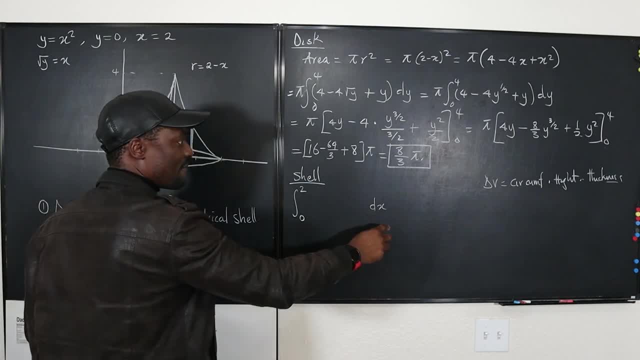 this is gonna be, okay? So we've already written that. 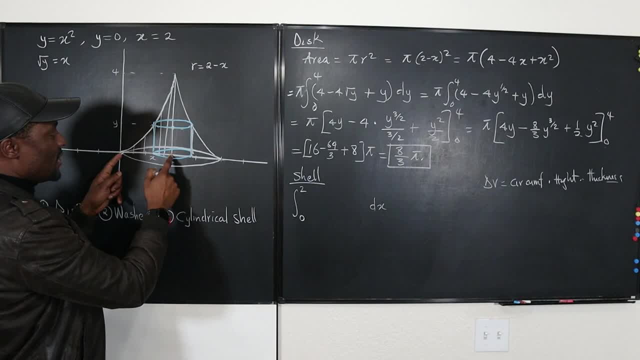 We also know that the boundaries are gonna be from the beginning to the ending of the original part that you rotated always. So we're ready to fix that. Now, the next thing to do is to determine what the height is. 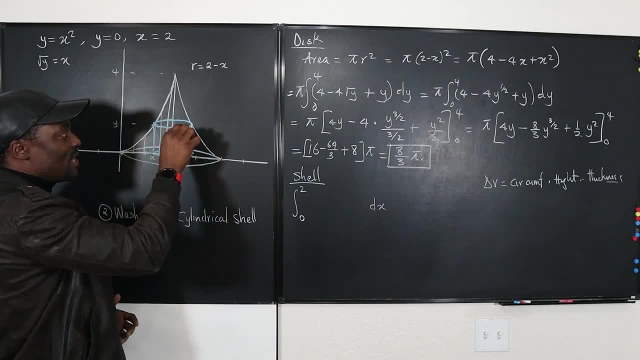 We can say by all means that the height is whatever you get here. 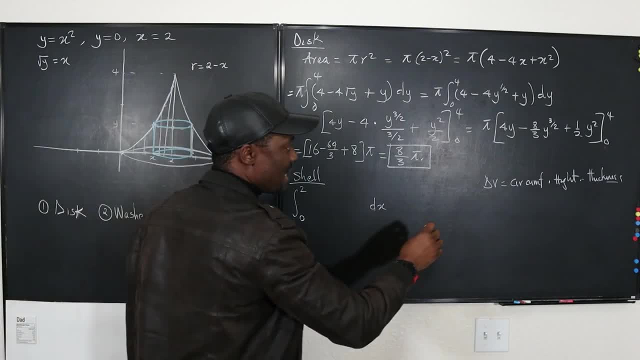 If you go higher, it's still the value of Y, okay? So the height is gonna be Y. This is gonna be DX. 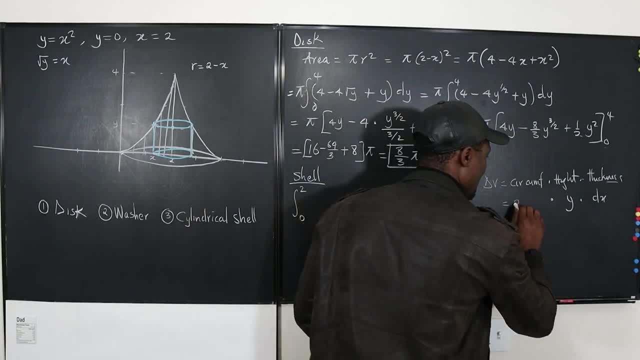 And now we need to find what the circumference is. Remember, the circumference is two pi R. 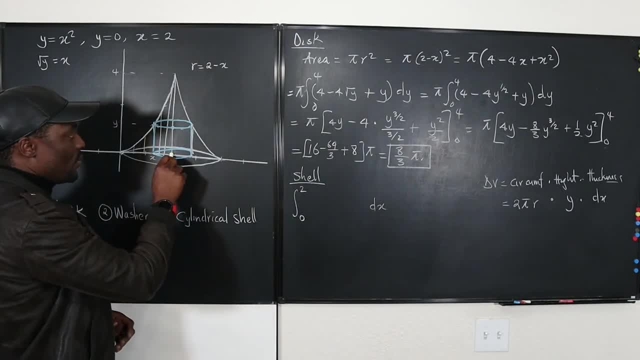 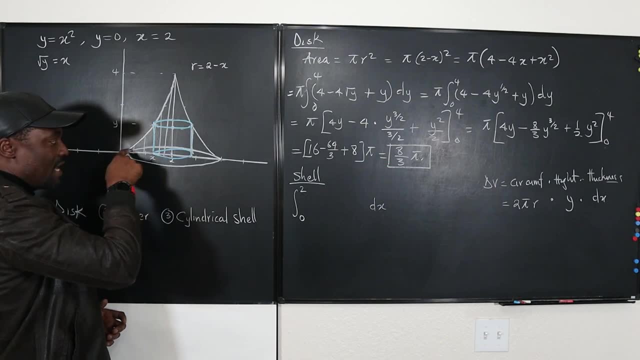 So what really is the radius of the cylinder? Well, remember, just as we did, because you're starting from, this is the center, it's gonna be the distance from here to any part of the cylinder you're dealing with. 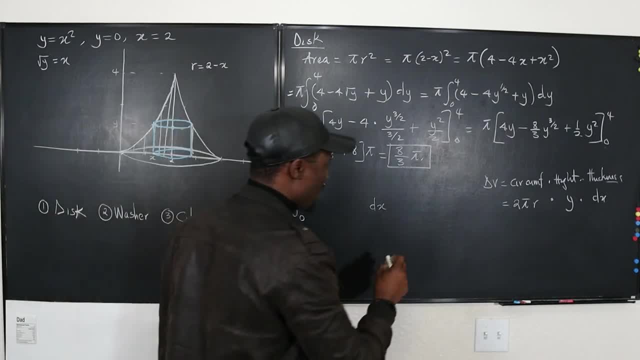 So it's still two minus X. So we're gonna say that this is equal to two pi. This is gonna be two minus X. 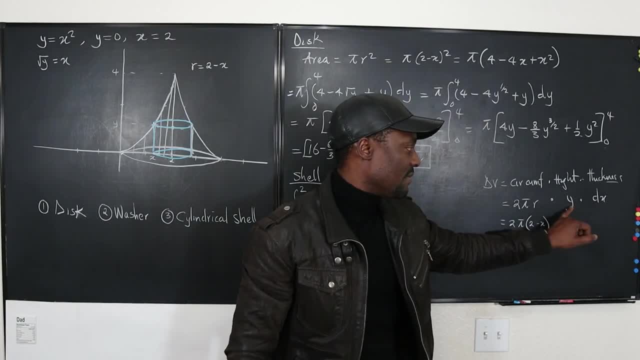 And we said we have to do it in terms of X. Therefore, our Y is gonna be two pi X. 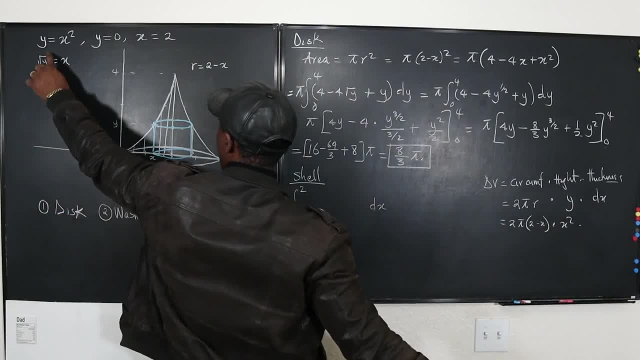 Y has to be X squared, or X squared. Y equals X squared, okay? 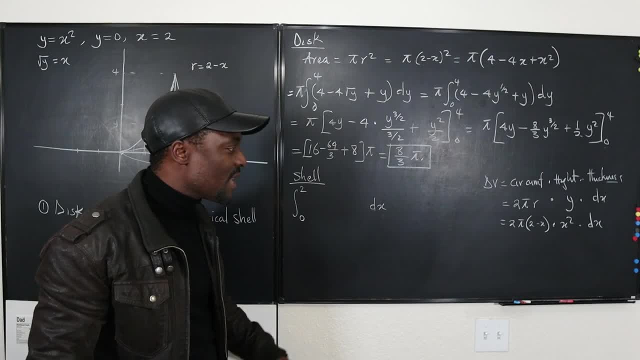 And then this is DX. So this is the setup for this second part. 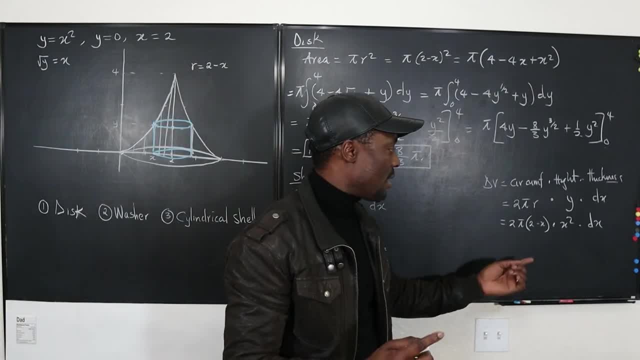 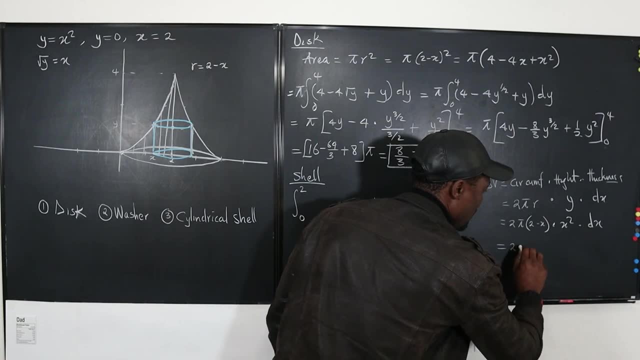 It could be a little tricky, but it's circumference two pi R times this times this. So if we clean this up, our DV is gonna be two pi times, 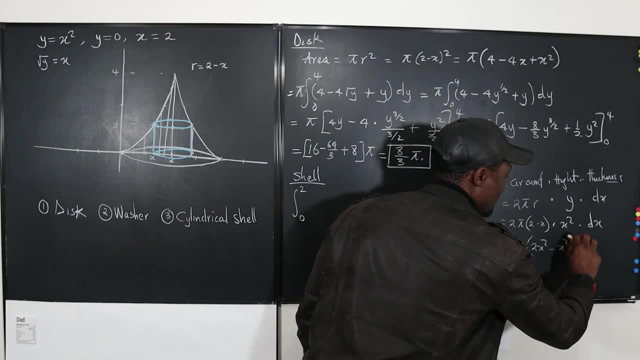 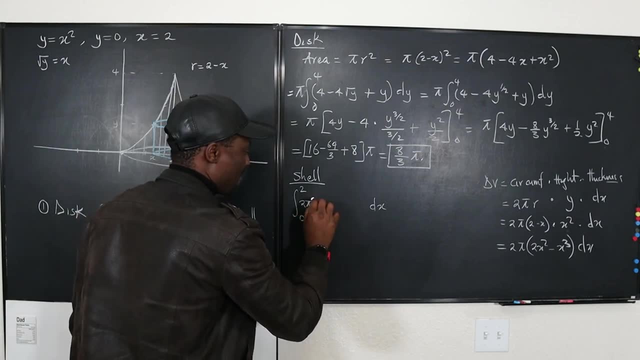 if we multiply this, you're gonna get two X squared minus X cubed DX, okay? And that's what I'm gonna bring in here. I'm gonna put the two pi on, okay, let's write everything. Two pi times two X squared minus X cubed DX. 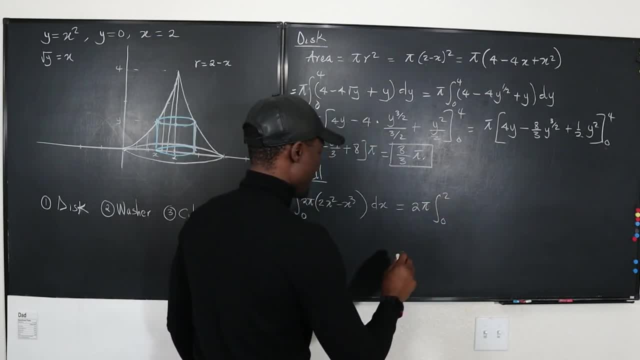 And we're gonna have zero to two of two X squared minus X cubed DX, which if we integrate, I'm gonna have two pi. 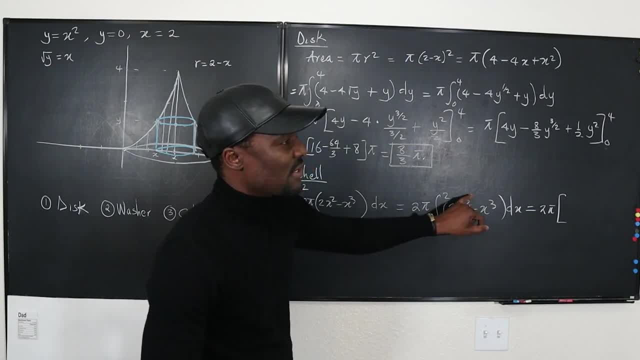 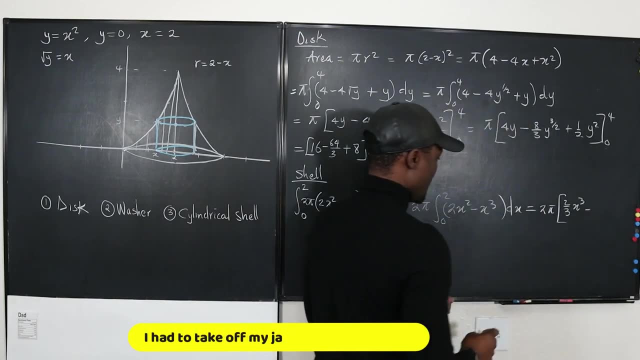 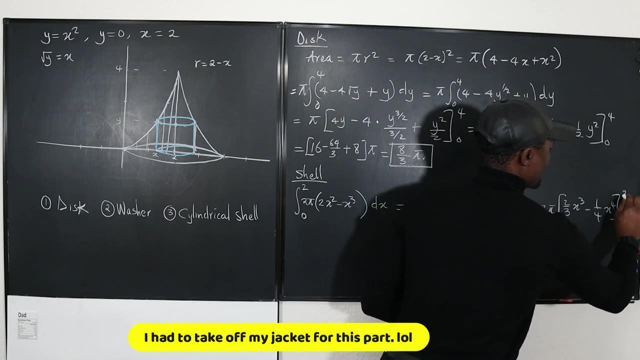 And on the outside, the integral of this is gonna be two times X cubed over three. That's two over X squared minus X cubed DX. Two over three X cubed. And then this is gonna be minus X to the fourth divided by four. That's gonna be one over four of X to the fourth, evaluated from zero to two. And because both terms contain X, the zero is gonna give me zero in either case. 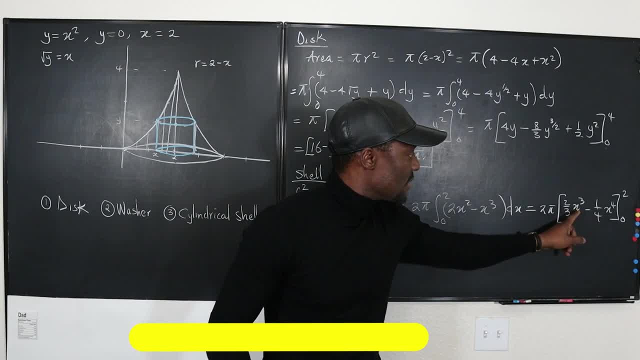 So I'm just gonna focus on the two. And then I put two here. This is gonna be eight. Eight times two is 16. 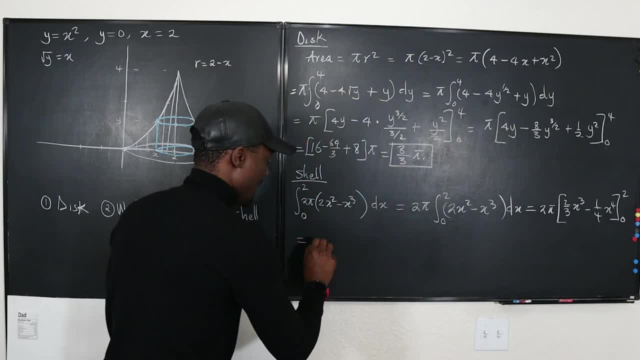 16 divided by three is 16 over three. Well, there's no way to hide.